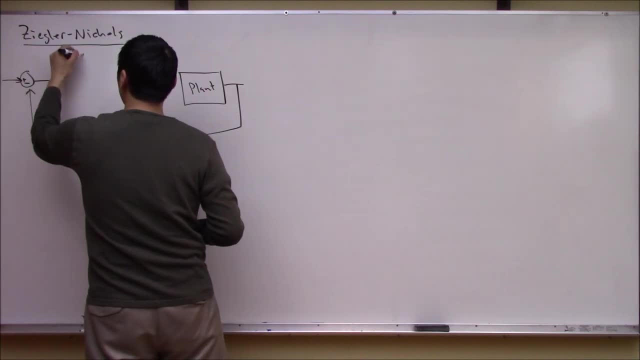 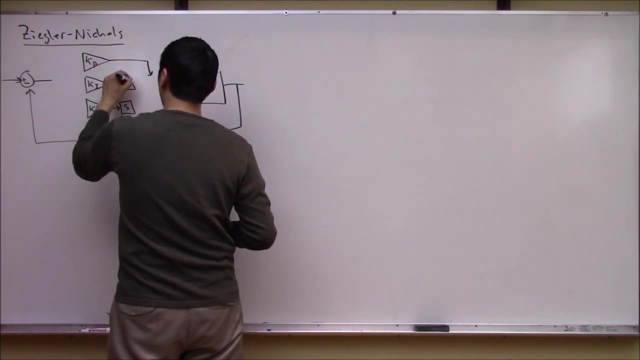 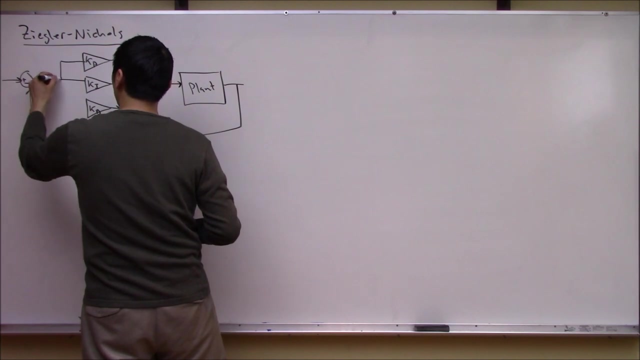 And the reason they're so attractive is because they're fairly simple to implement and understand, Because one reason, primarily, is that they are parameterized by only three values, namely a proportional gain, an integral gain and a derivative gain, So there isn't a whole ton that goes on with a PID controller. 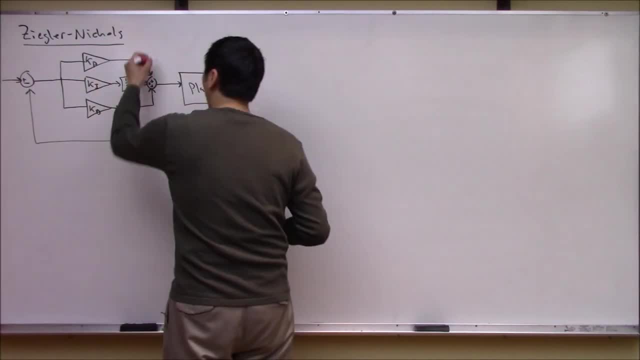 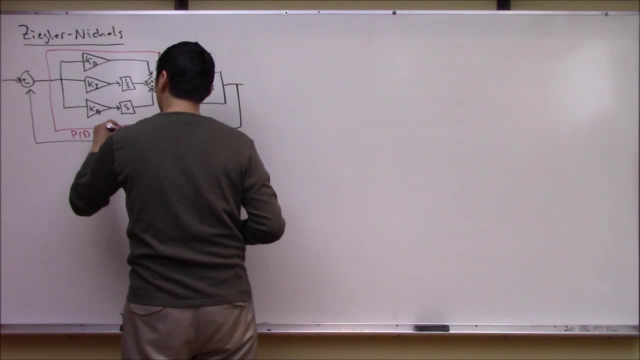 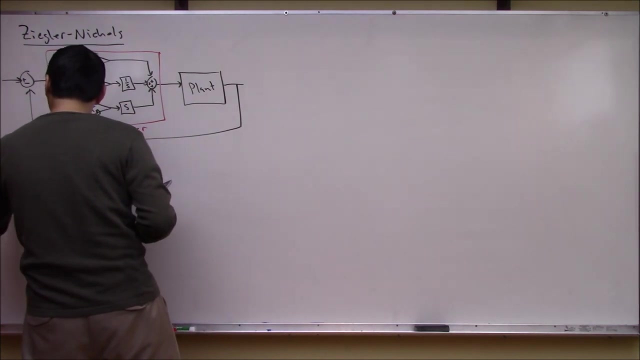 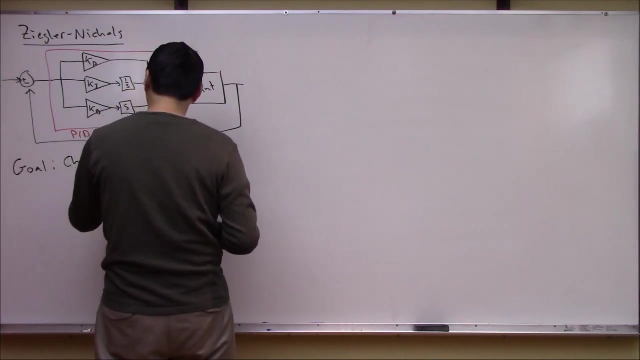 So the architecture is pretty simple and you see that again, your job as a control systems engineer, when you're trying to design this PID controller, is really just to pick these three values of Kp, Ki and Kd. So, on a very simplistic level, the goal as a control systems engineer is to choose Kp, Ki and Kd in a quote-unquote appropriate fashion, or choose them appropriately. 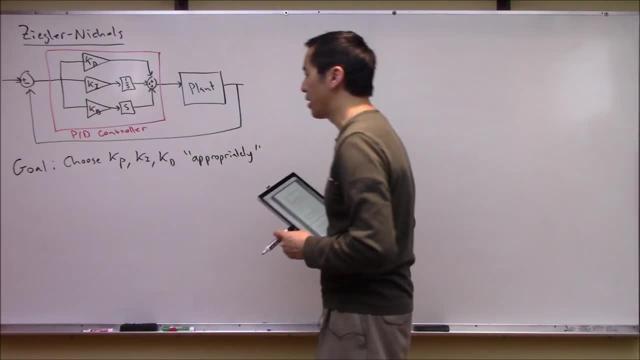 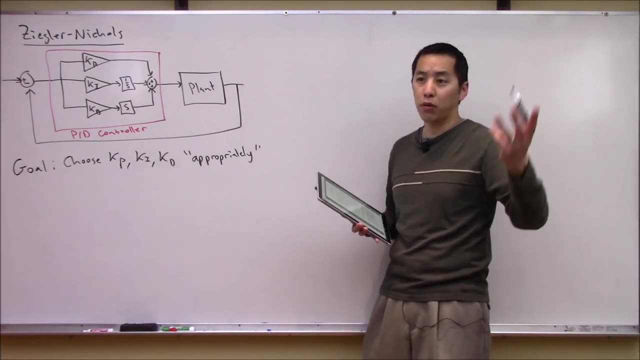 We'll talk a little bit more about what appropriately means, maybe in a future lecture. but on the surface this actually doesn't look like that hard of a problem, right? All you need to do is pick three values, Pick three of these real numbers, and then you can go off to lunch. 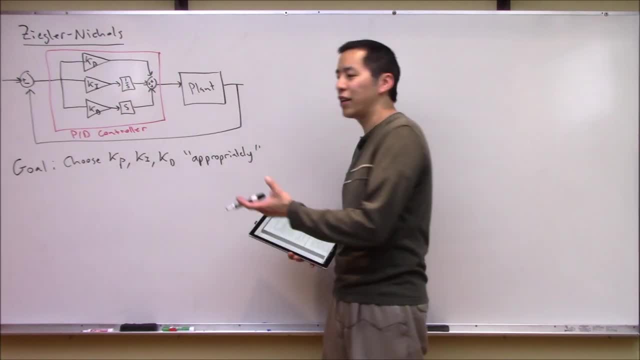 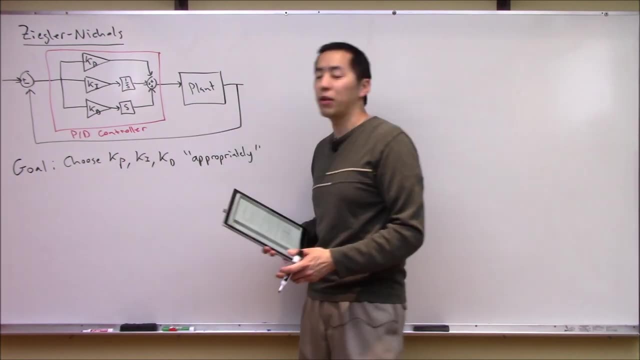 But in practice, right. you don't want to just be simply shooting in the dark and just shotgunning Kp, Ki and Kd values and seeing and crossing your fingers and hoping it works right. For example, what if this system, this plant you're controlling, is very, very expensive, like a rocket or a satellite? 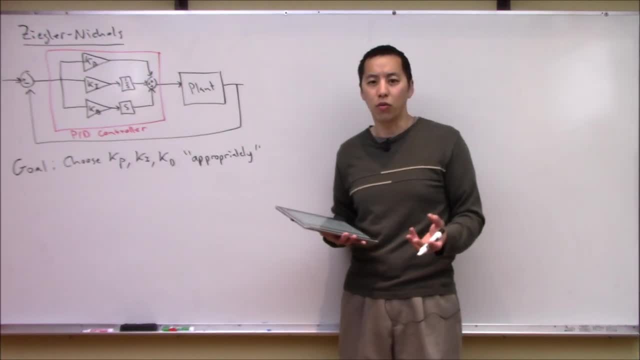 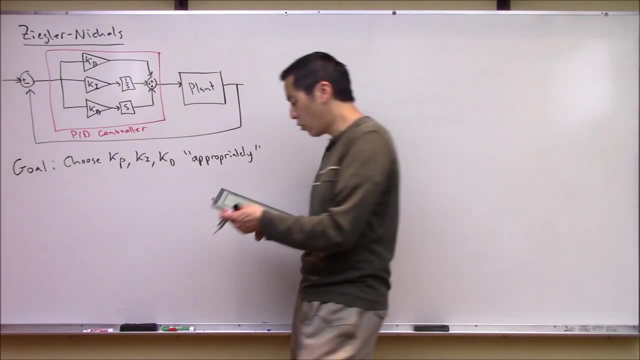 Well, you probably need a more intelligent way to get the Kp, Ki and Kd values. So Ziegler-Nichols is one technique that's going to allow you to do this in an iterative online fashion, So maybe we should write that down. 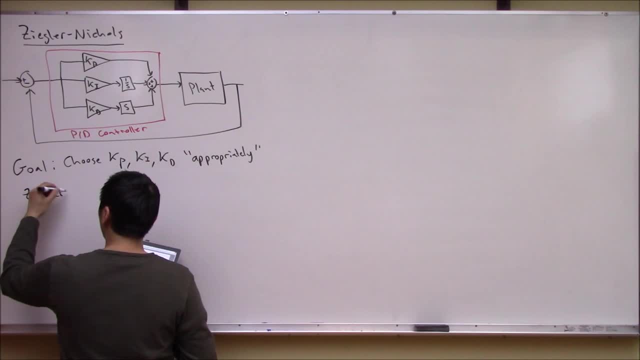 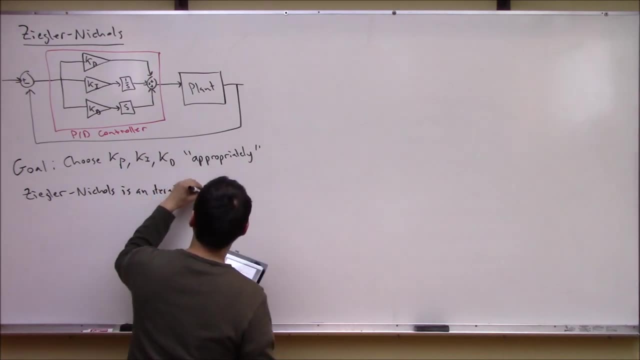 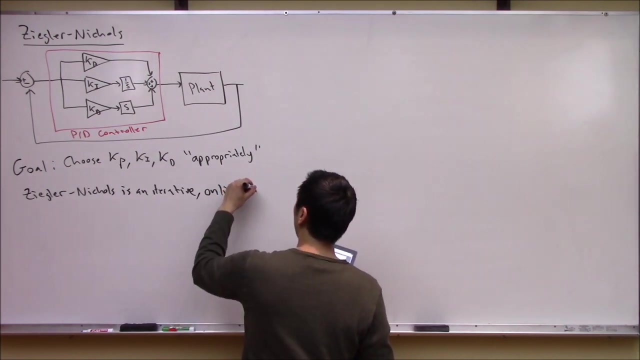 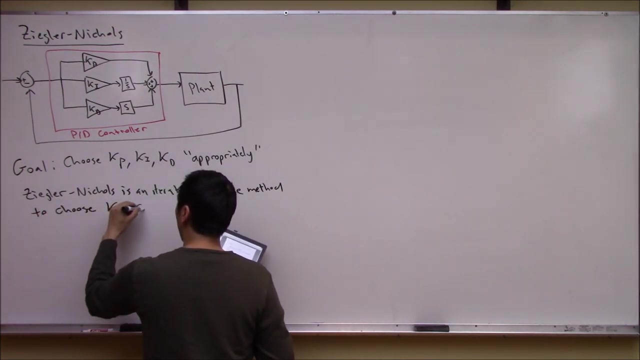 So Ziegler-Nichols- let me put this on the board- is an iterative online, meaning we can do this directly without needing a model here. So it's an iterative online method to choose these values of Kp, Ki and Kd. 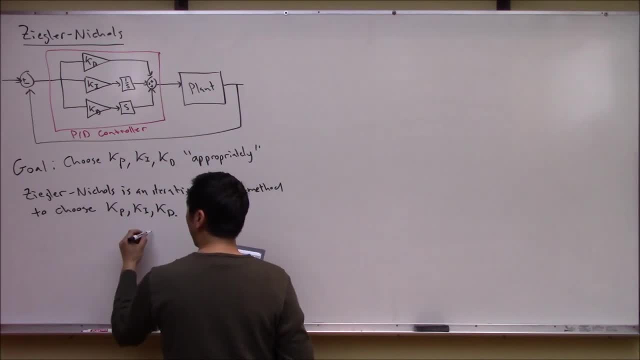 So what the method will produce is three values. So we're going to go into the algorithm a little bit later, but maybe let's just write it like this: So Ziegler-Nichols procedure- And I think procedure is maybe a better word than algorithm- because we're going to see you have to do a couple of steps- 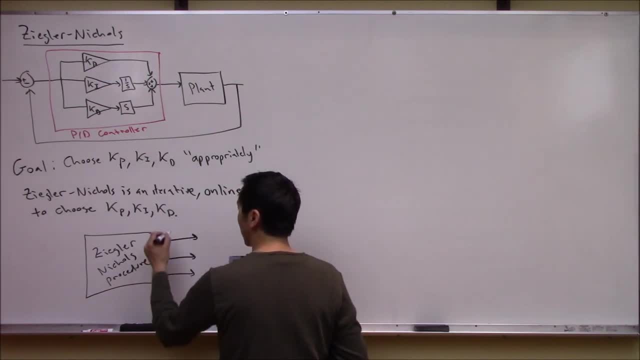 But at the end of these steps, what you're going to get out are three numbers. You're going to get Kp, which is definitely the proportional control that we're looking for, But you'll also get these other two sort of time constants. 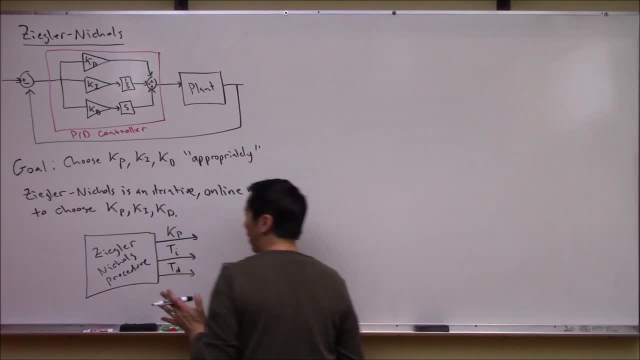 Let's call it a Ti and a Td. So if you read a lot of older literature about Ziegler-Nichols, this is what it says it produces. It gives you these three numbers, And what it tells you then to do with these three numbers is: you can then compose a control law that looks like this: 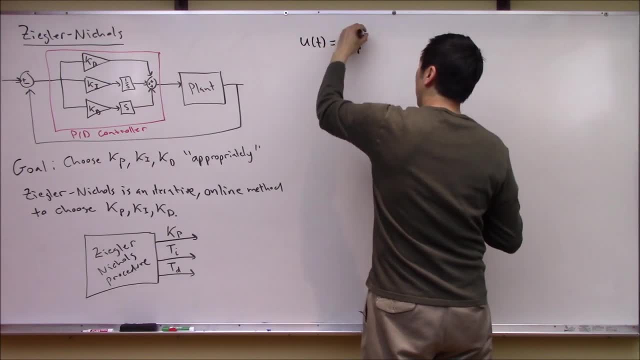 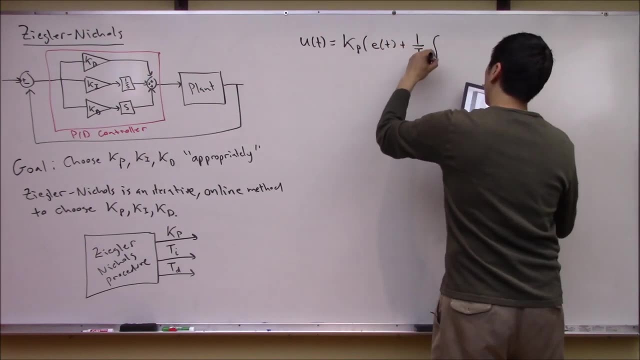 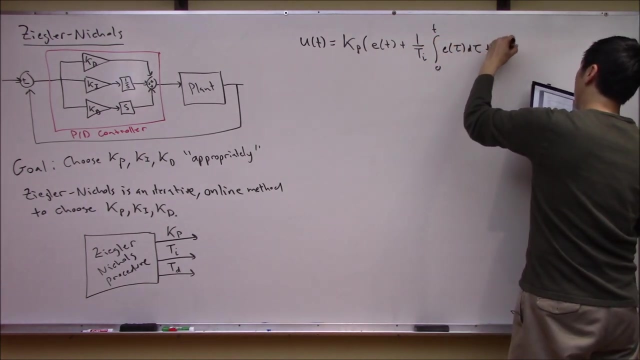 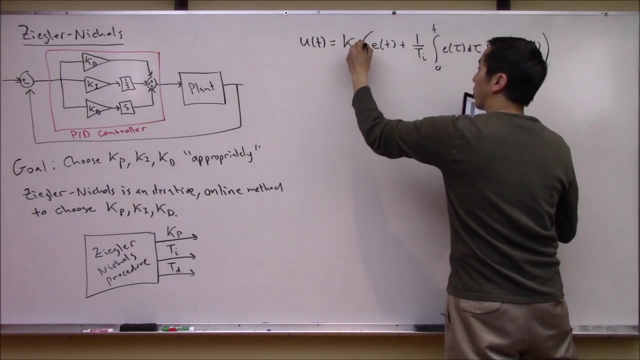 You can get: U of T is equal to Kp times E of T plus 1 over Ti. integral from 0 to T of E of tau, d tau plus Td times dE of T dt. I'm going to put an end parenthesis here to close this parenthesis. 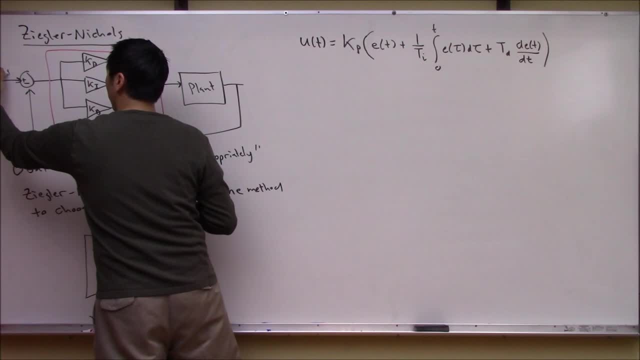 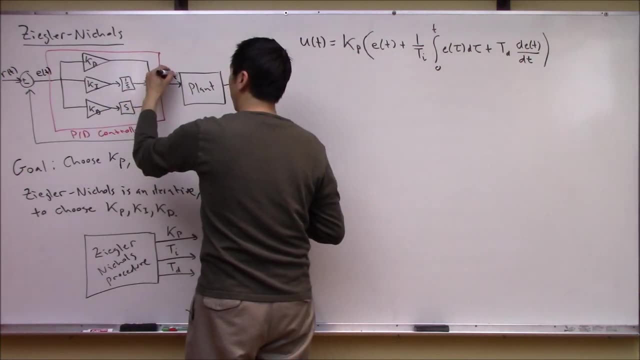 Maybe we should label, I guess, in this picture: here's your reference, Here's your output, And then here is the error, And then here's the control U of T: Right, Your standard architecture. Okay, so this is the control law that it says you should implement. 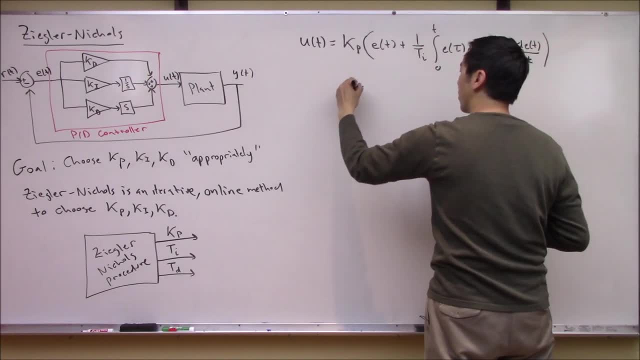 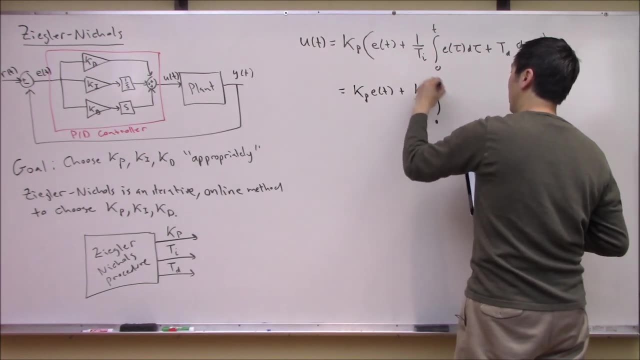 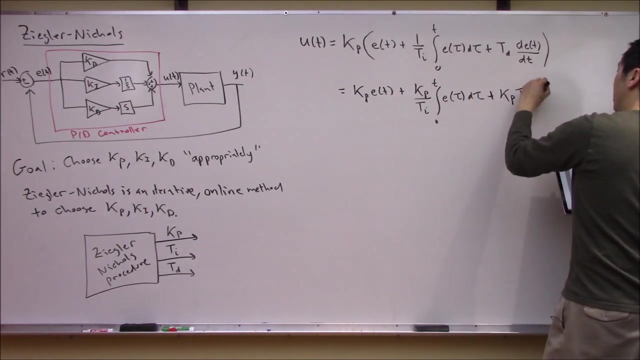 Well, if you distribute this Kp through, you see that this is Kp times E of T plus Kp over Ti times integral 0 to T. E of tau d tau plus Kp times Td, dE of T, dt Right. 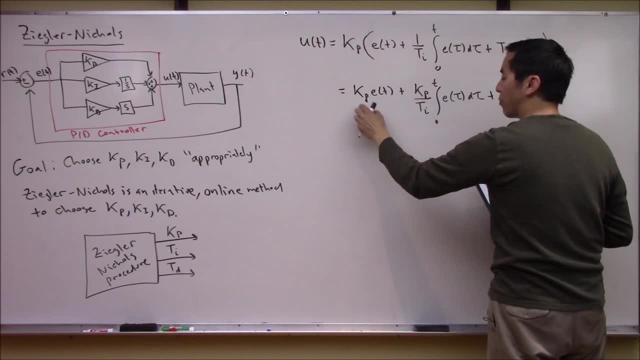 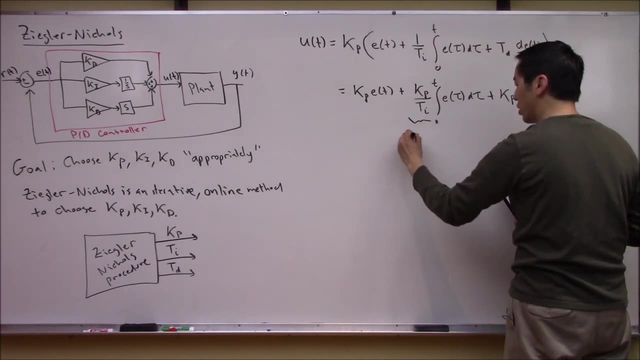 So again it says the control is the error times some number. so this is definitely your proportional gain plus the integral of the error times some other number. So this quantity right here is actually your Ki Right And similarly over here here's you have the derivative of the error. 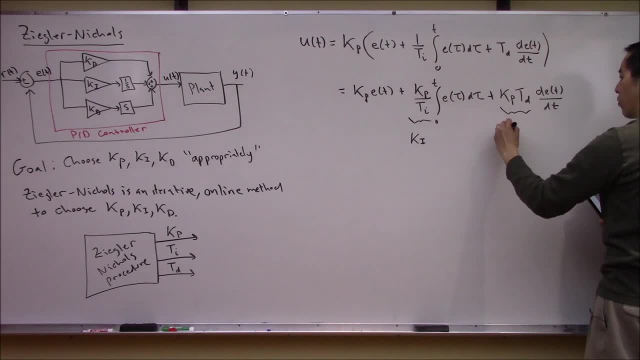 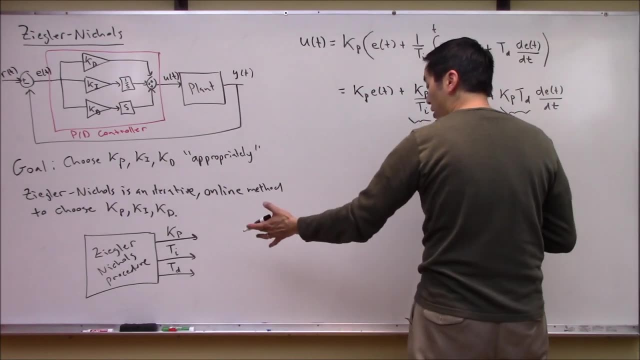 and you have some other constant in front. So this entire product here is what we think of as our traditional Kd value, So in other words, Ziegler-Nichols. the alternative way you could think about this is: okay, Ki is just going to be Kp all over Ti. 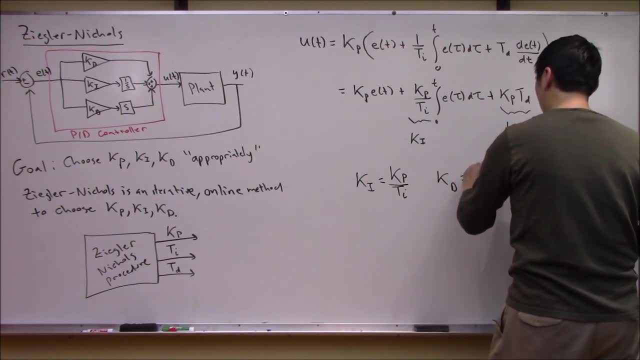 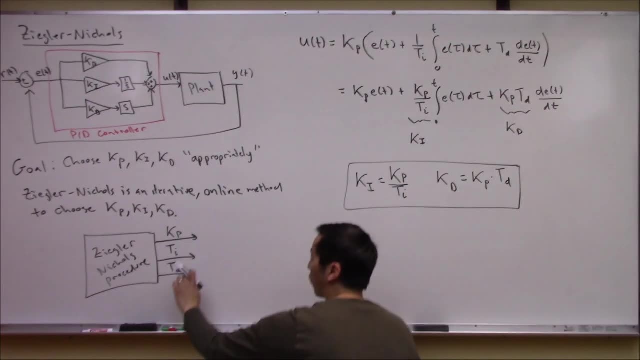 and Kd is just going to be Kp times Td, Right? So these two equations you could actually use to transform Ti and Td, I'll just say these equations. Maybe we should have labeled them In my notes. I call these equations 3 and 4.. 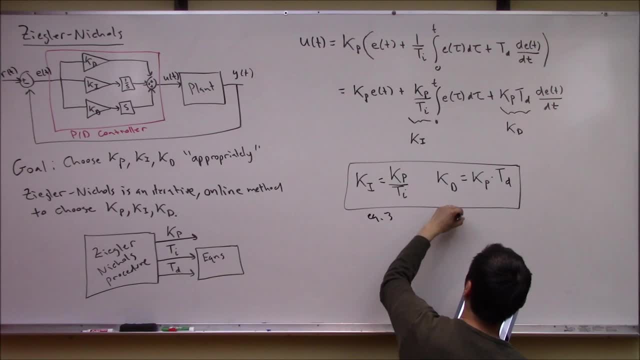 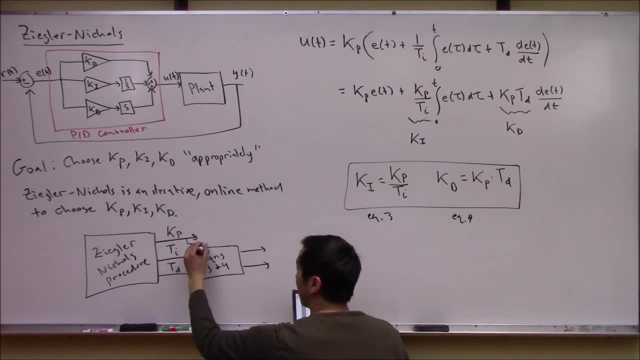 So this is equation 3, and this is equation 4 in my notes. So equations 3 and 4.. You could also use this to translate and I guess technically you actually need Kp here, But you could get Ki and Kd. 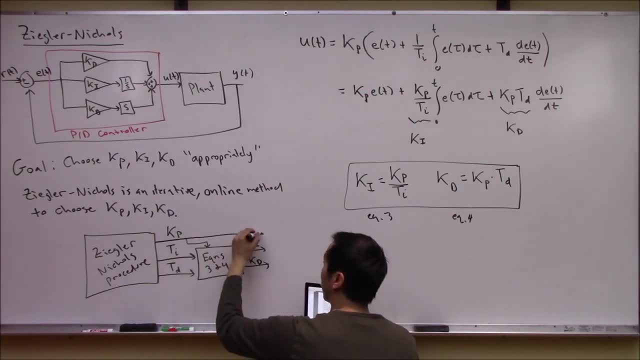 So the other way you could think about this is that, again, Ziegler-Nichols will also yield Kp, Ki and Kd. So a lot of forms and a lot of tables you're going to see in a second. 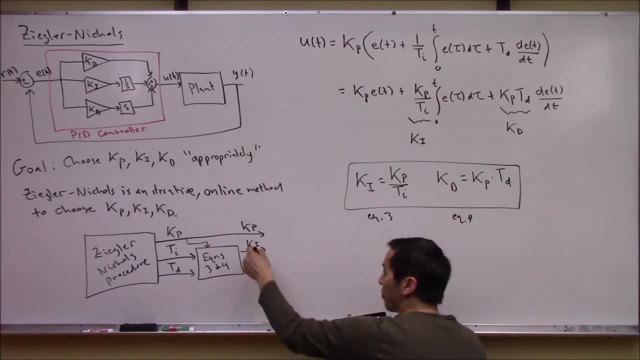 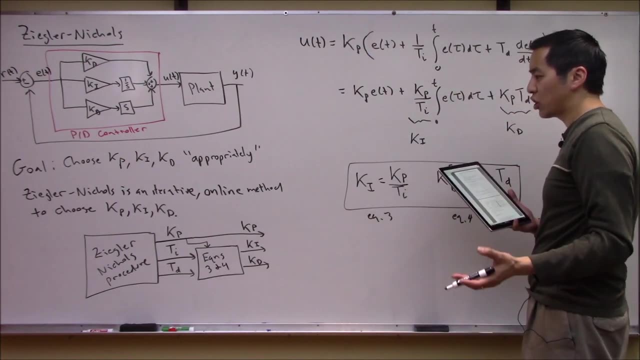 Sometimes they list Ti and Td as the output of the Ziegler-Nichols method. Sometimes they list Ki and Kd. Okay, So let's talk about the procedure for Ziegler-Nichols. It's actually not that bad. 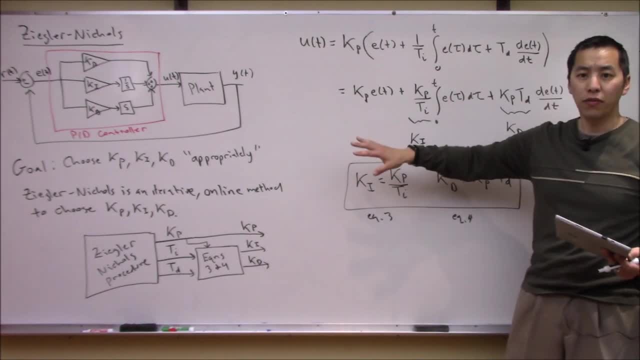 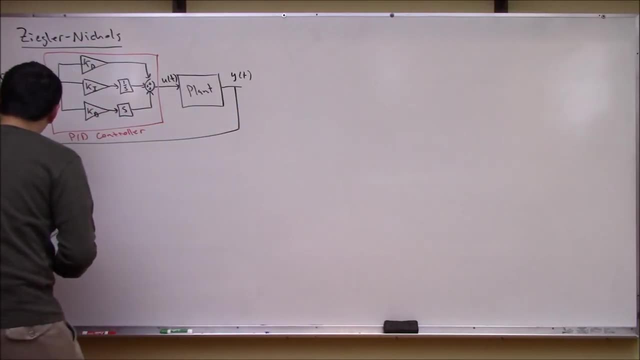 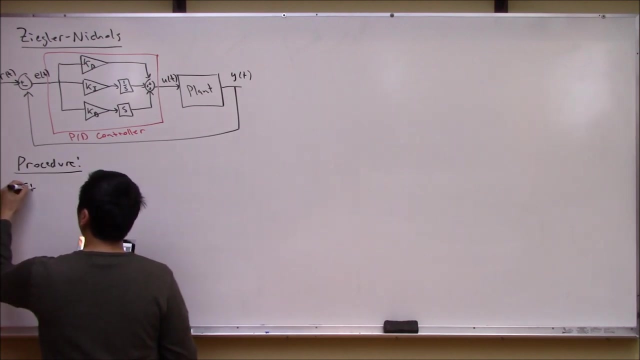 So tell you what? Give me a second, I'll pause the video, erase the board and let's list out the algorithm and the procedure. Okay, So the Ziegler-Nichols procedure is actually pretty straightforward. So the first thing we're going to do here is start with Kp equal to something small. 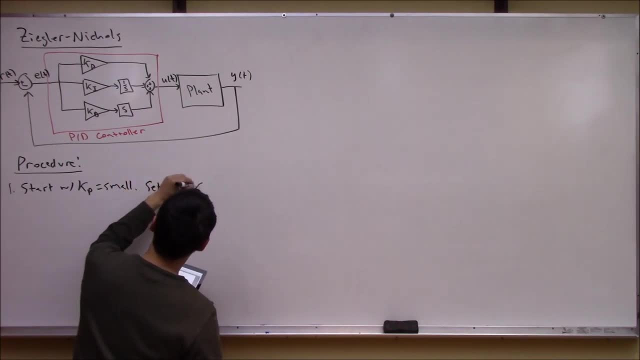 and set the Ki and the Kd to be 0.. Okay, So basically, in this situation, you knock out the integral and derivative and you only have a proportional controller controlling the system. Okay, And then what you're going to start doing is: 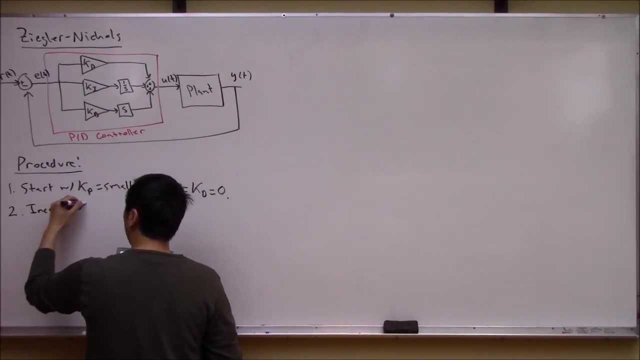 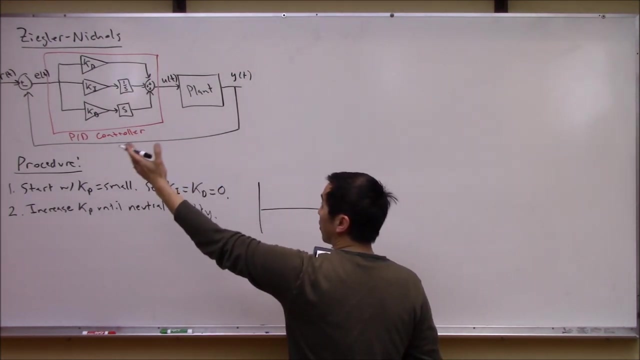 you're going to start increasing Kp until you achieve neutral stability. So what that means is you're going to take your system and you're going to perturb it, and hopefully it's trying to hold a reference of, say, 0 using only this proportional controller. 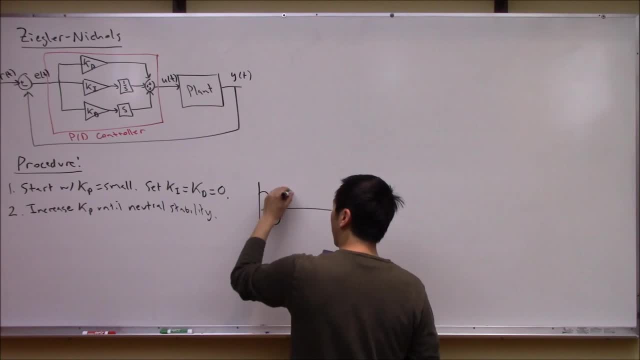 And you reach neutral stability when you perturb it and the system oscillates and the oscillations neither decay back to 0 nor explode Right. So you want to make sure you have neutral stability. So this is what you're gunning for. 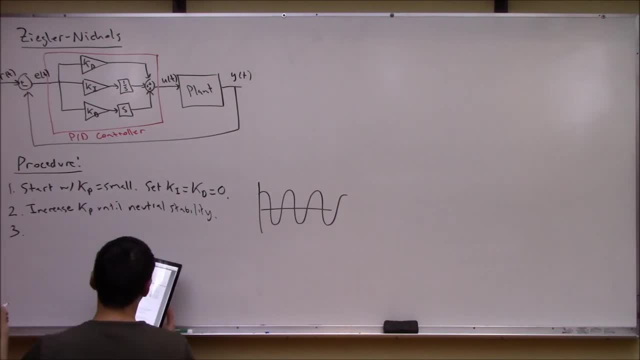 Okay, So once you achieve neutral stability, you're going to go ahead and record what is called the critical or the ultimate gain, Ku, which is just this Kp at neutral stability. So, whatever Kp you used to get this neutral stability or stability situation. 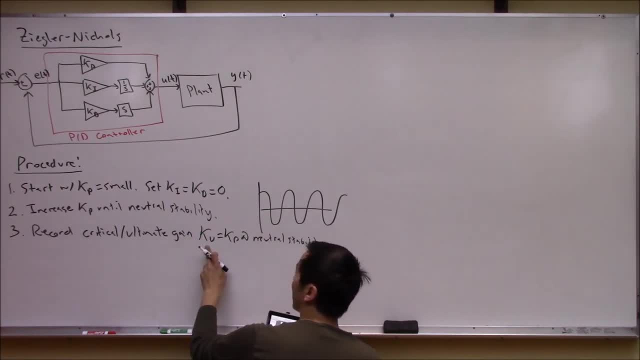 just call this Ku, this ultimate gain. And also, not only are you going to get the gain, but you're also going to record the critical slash, ultimate period of oscillation, And let's call this Tu. So again, the picture goes along here. 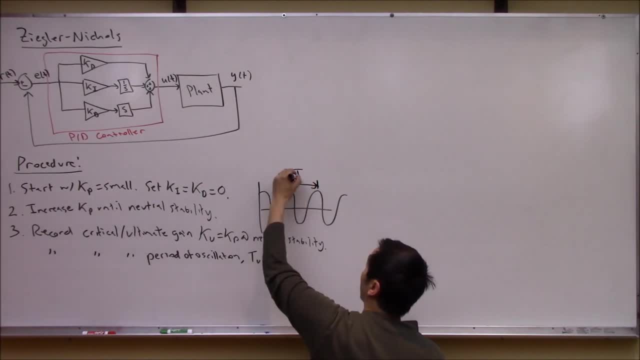 is. you just want to find the period of this oscillation and call that Tu in seconds, Right, Okay. So once you have both of those two parameters, Ku and Tu, what you can then do is look up the associated Kp, Ti and Td. 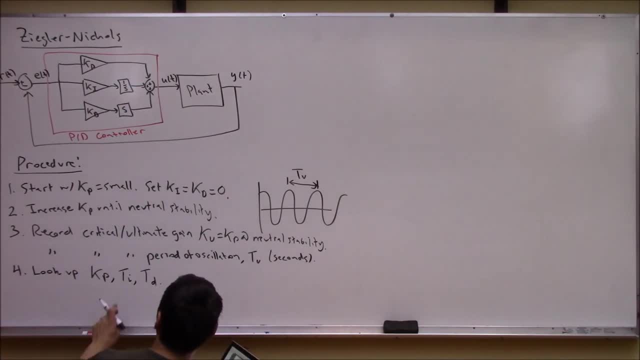 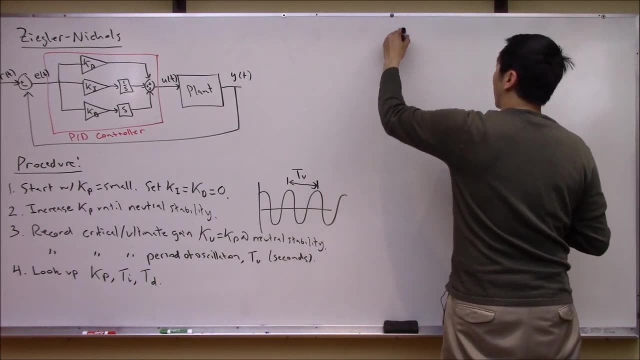 Right, Those three parameters from the Ziegler-Nichols. So this is something that people have derived and you can find it in a table that basically says: all right, here's the Kp, here's the Ti and here's the Td. 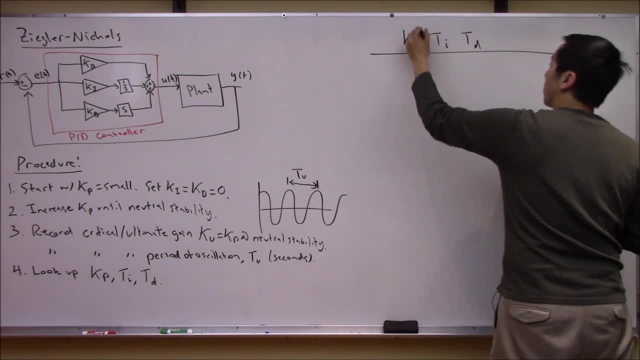 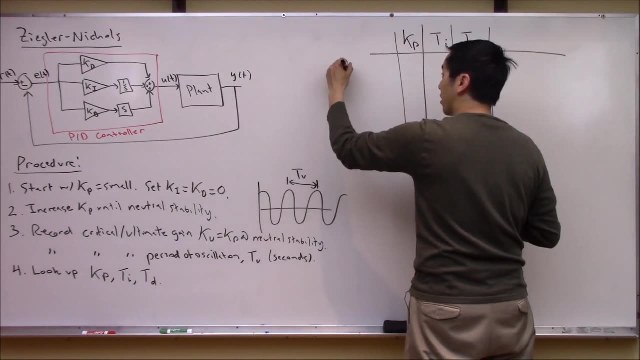 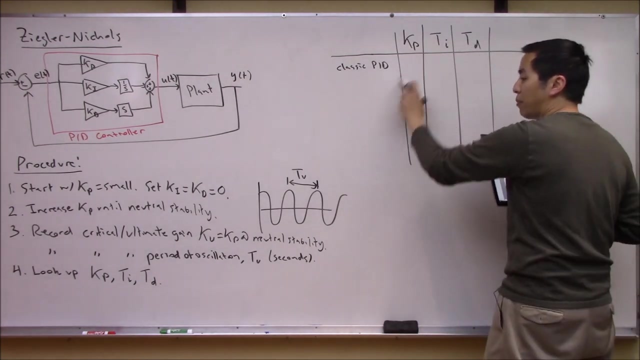 And here's the Td values. And in this case, if you are just doing, let's say, classic PID, right, That's the whole point of Ziegler-Nichols. You want to just find the PID gains? Well, the way you find Kp is you take Ku. 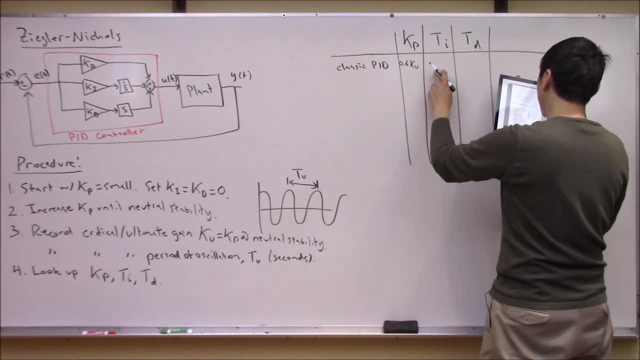 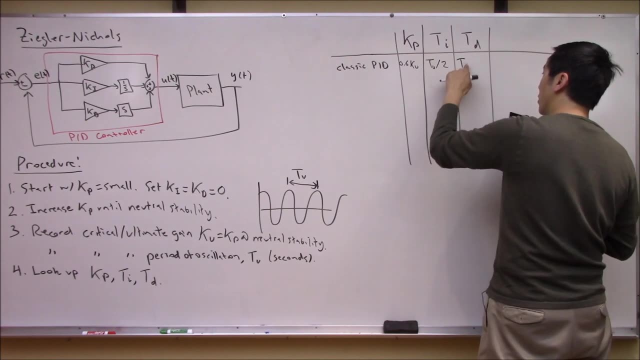 and you multiply by 0.6.. The way you get Ti is you take the period of the oscillations and divide by 2.. The way you get Td is you take the period of oscillations- sorry Tu- and divide by 8.. 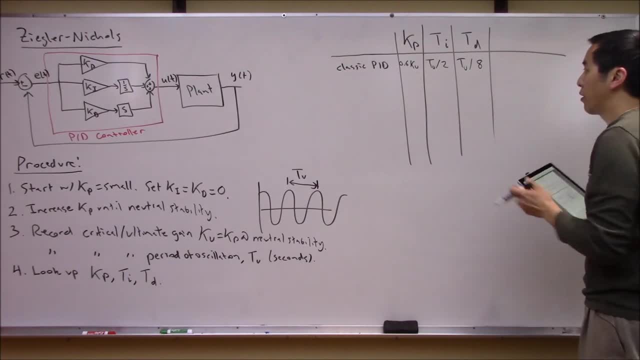 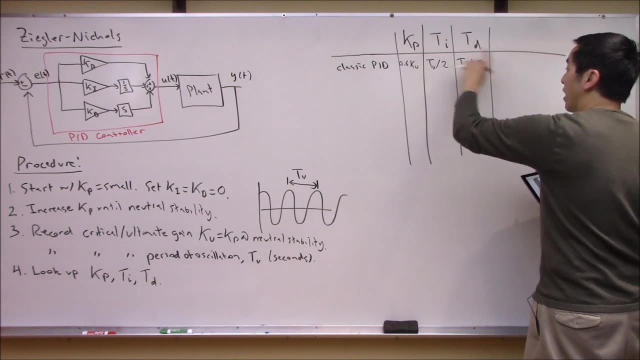 So it's just a formulaic lookup at that point right. People have already established these relationships between the ultimate gain and the period of oscillations to get you the Kp, the Ti and the Td. Now these numbers for Kp, Ti and Td could change. 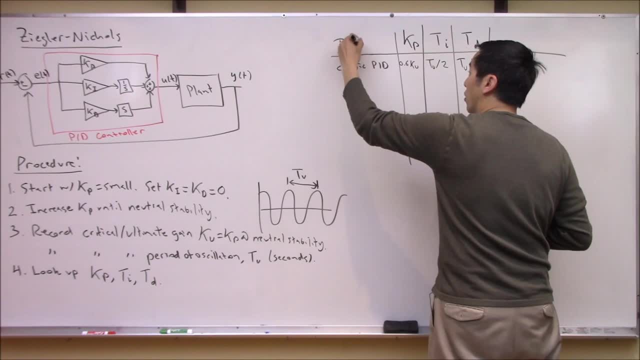 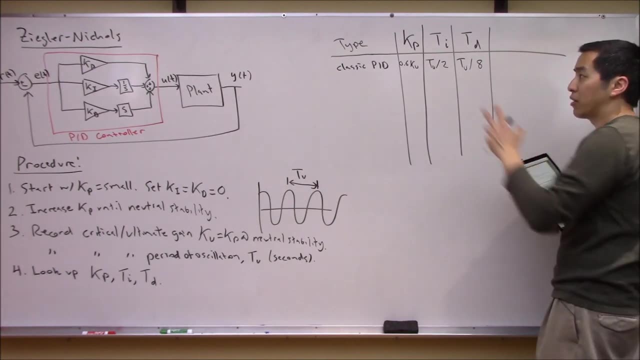 depending on what type of control scheme or performance you're looking at. So 95% of the time I think you'll see these numbers spit out or this relationship, because you're just doing normal PID. But people have also done things for, say, 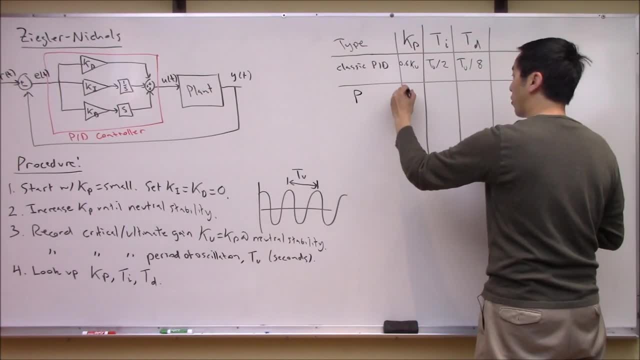 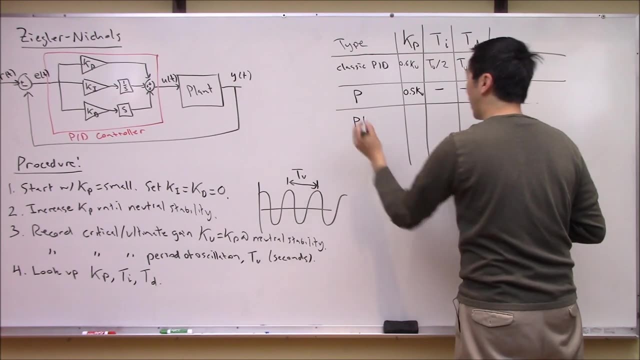 just plain old proportional control. So in that case you would use 0.5 times Ku, and these two are not applicable. You could also do say just Pi. So in this case just Pi would be 0.45 Ku. 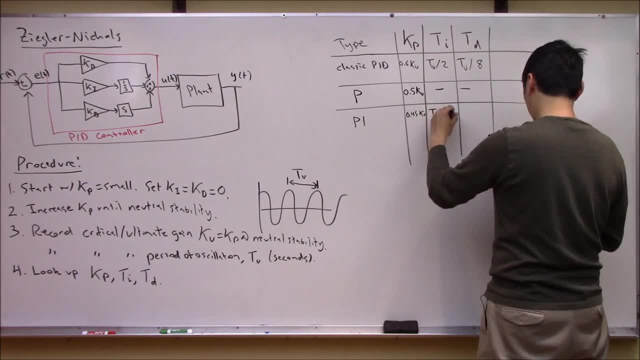 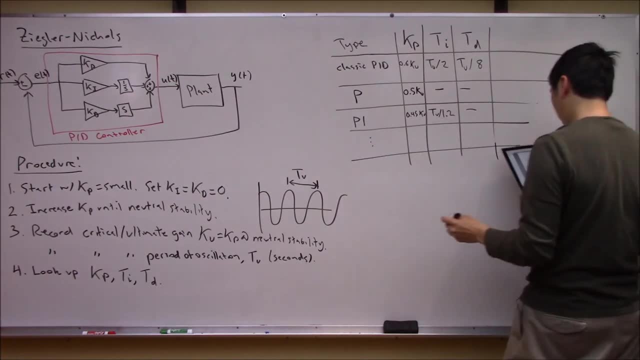 and then this would be Tu over 1.2, and this is not applicable, and et cetera, et cetera. right, There are different schemes and different relationships for different types of controls. Maybe let's do one last one. 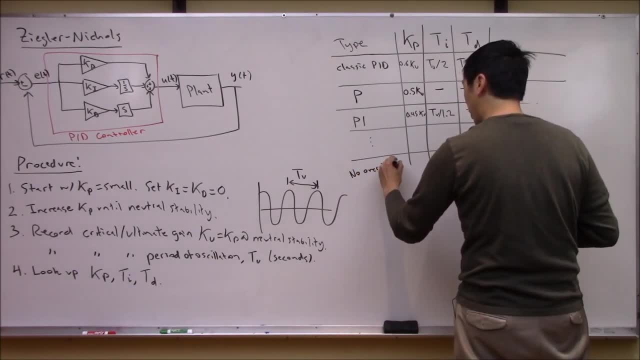 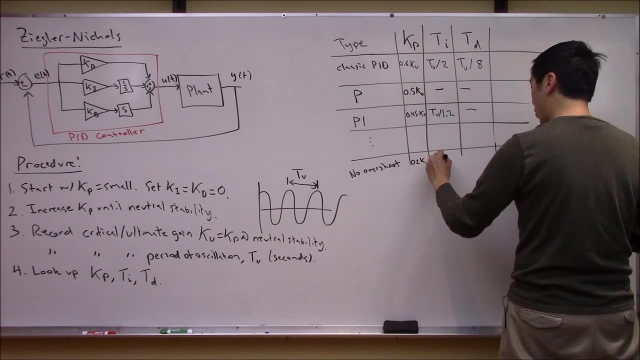 How about, if you want no overshoot? So in the majority of cases, if you use a Kp of 0.2 times Ku, so really back off of that gain. and you use Tu over 2 for the Ti variable and then you finally use Tu over 3 for the Td variable. 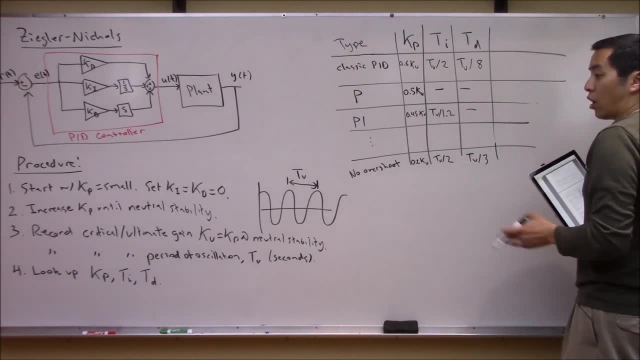 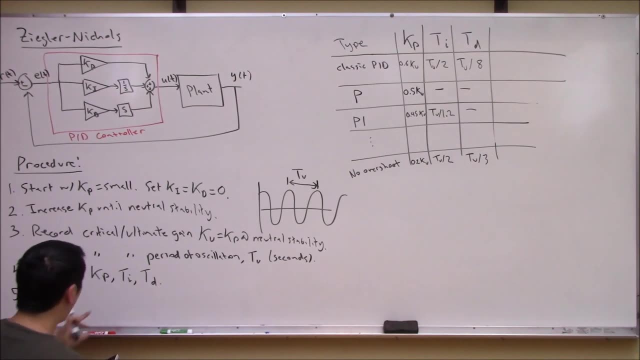 hopefully that gets you no overshoot. okay, So let's, maybe There's one more step that we could do here. So, like we said earlier, I personally don't like thinking about Ti and Td. I really like thinking about these three gains. 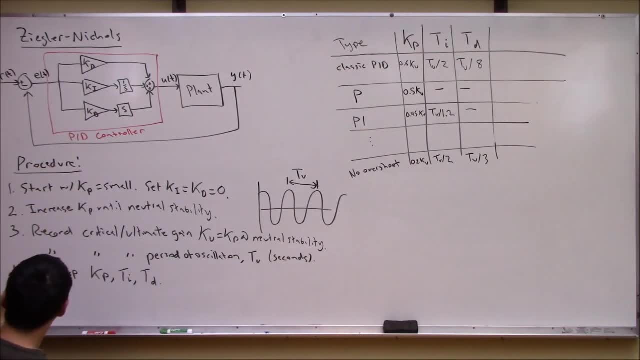 Kp, Ki and Kd. So what you could do in step 5 is you could compute the Ki, gain and Kd from. what we called earlier was, I think we said, equation 3 and equation 4.. It's how we had labeled those right. 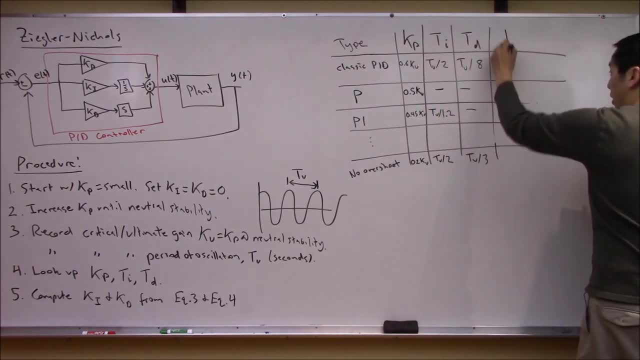 So what you could do is you could augment this table- Maybe I'll make another two columns on the far side- and you could basically get Ki, which I think we said the formula for that was. it was Kp divided by Ti, And you could also compute the derivative gain. 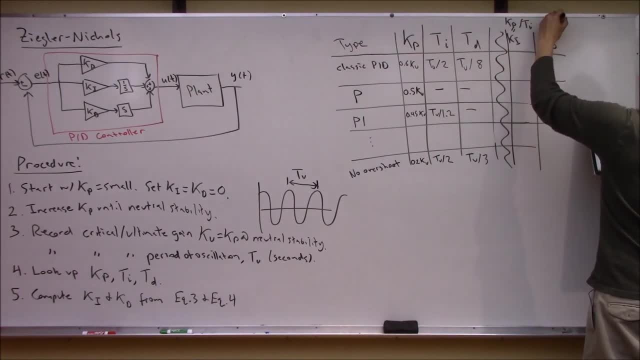 which we said was Td times Kp, right? So in this case, I think if you just did this math, you'd come up with 1.2 Ku over Tu and this one would be 0.2.. This one would be 0.075 Ku times Tu. 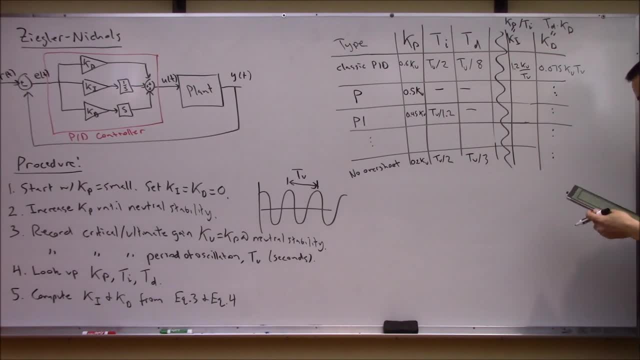 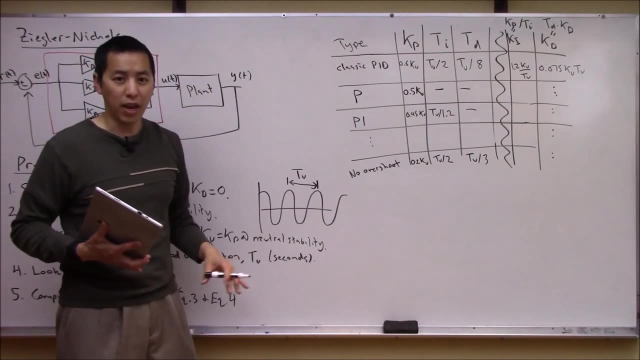 and et cetera, et cetera. You could fill out that relationship for all of these different parameters. So, in fact, instead of me writing out this table and maybe making errors and making it hard to read here, why don't I just go ahead and flash up the completed table? 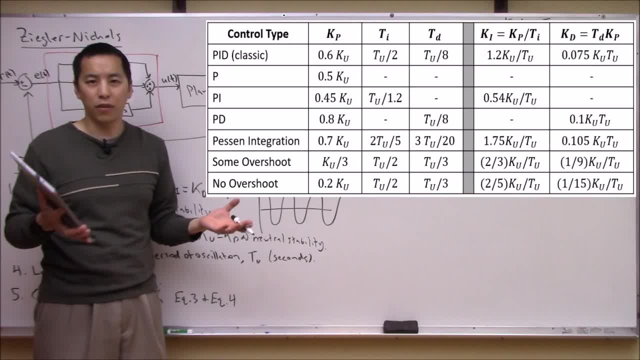 that I've typed up and written down in a nice fashion, So that's hopefully what you should be seeing on the screen right now is a nicer version of the table we were trying to draw. So, with that being said, now that we have the procedures set up, 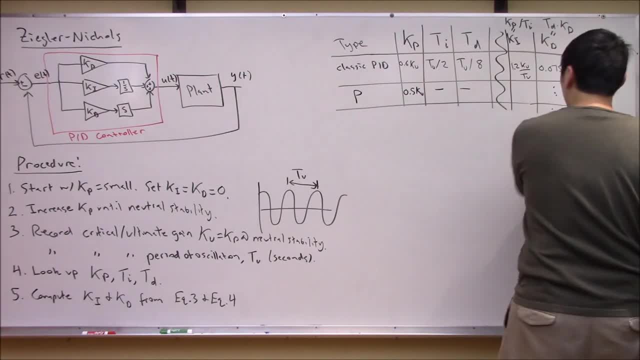 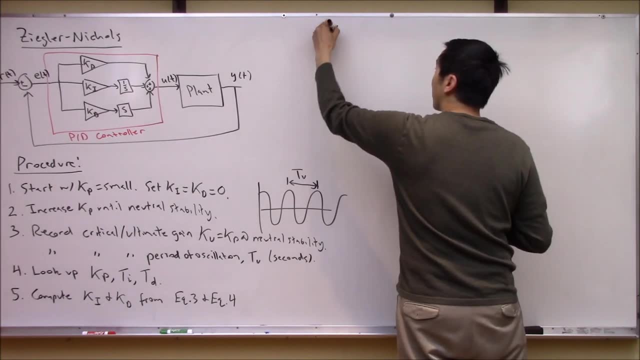 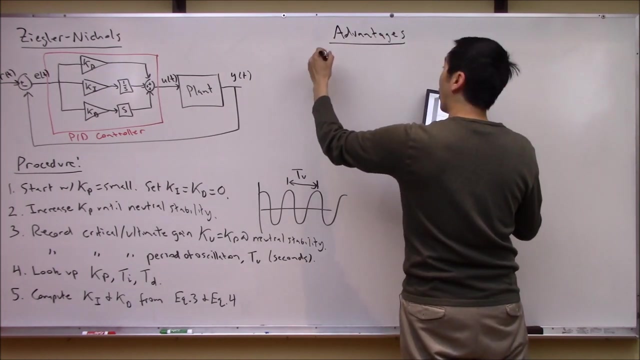 I think what might be helpful is let's talk about some advantages and some disadvantages of this Ziegler-Nichols technique. So obviously, some advantages or pros of this technique. here is well, first off, if you look at this, it really doesn't require a lot of understanding. 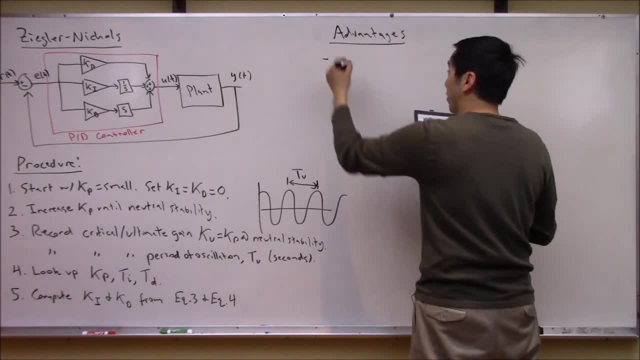 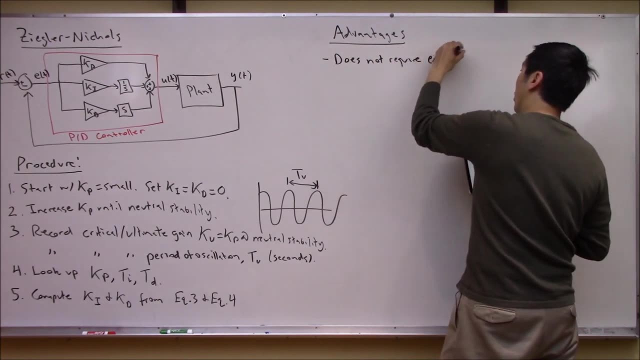 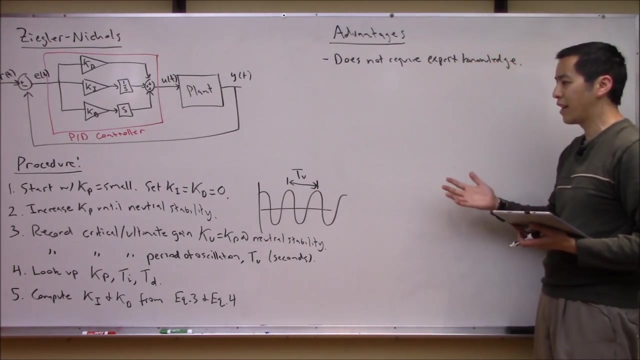 of control systems or dynamic systems. So let's just write down: does not require expert knowledge. It's basically a formulaic five-step process where you walk through it and nothing in here says you need to have a master's degree in control systems or differential equations. 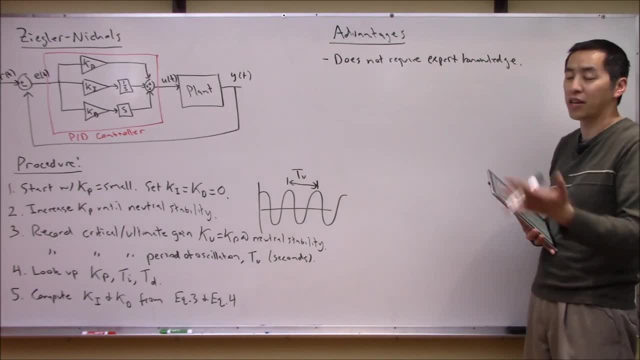 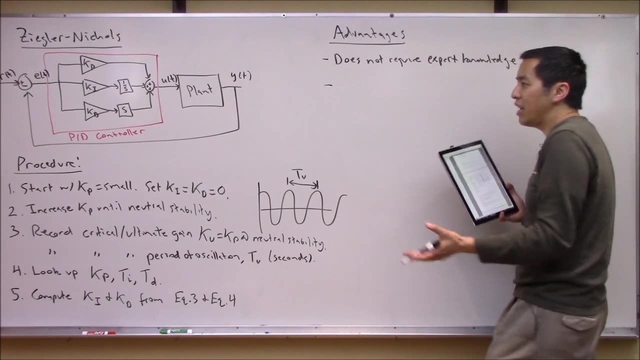 You just walk through these five steps and it will spit out a Kp, Ki and Kd that you can try on your system. Sort of related to this is also, you know what? you don't even need a differential equation or any kind of model for the plant at all. 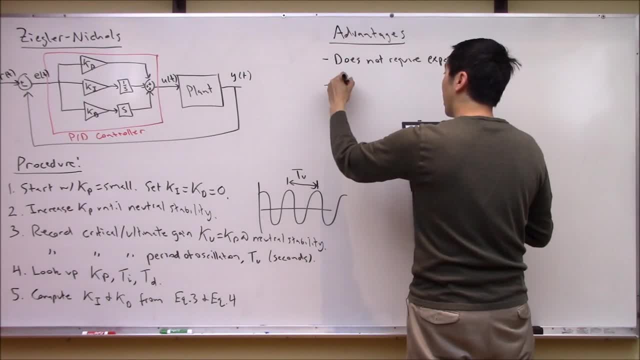 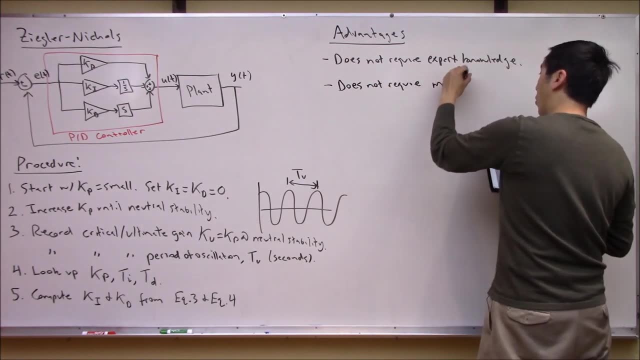 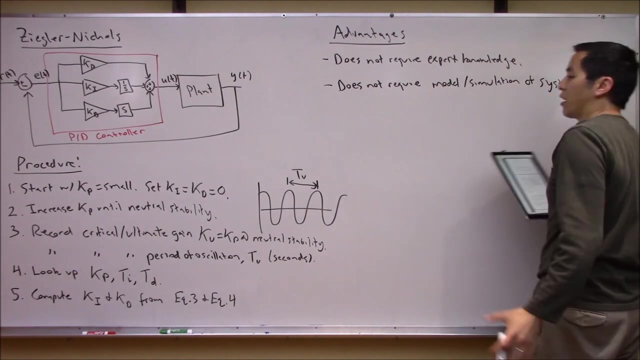 So here we can say that an advantage is it does not require a model or even a simulation of the system, So you don't need to know anything about simulating If you've got the piece of hardware sitting there in front of you again. 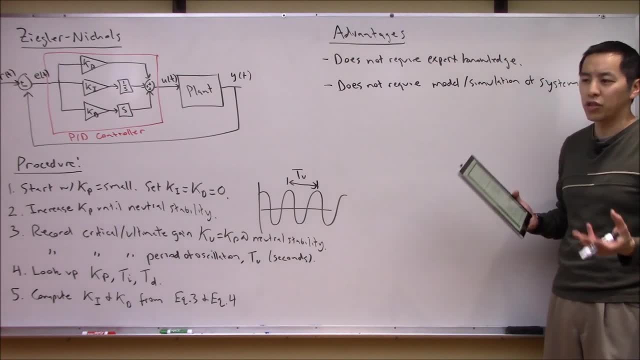 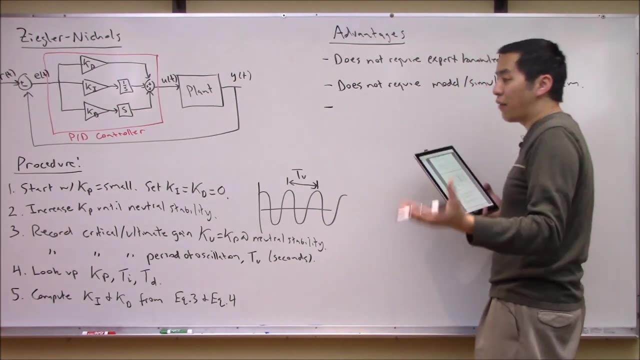 you don't need to know anything about ODEs or simulation or anything. Just run this procedure on the actual system. okay, And the other. the main advantage of this here is that it often produces a reasonable set of gains here, and it's a good point for starting. 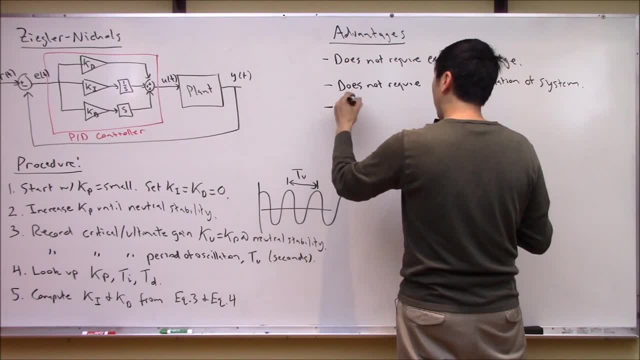 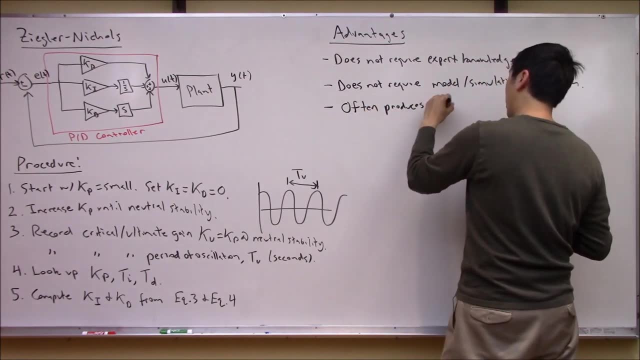 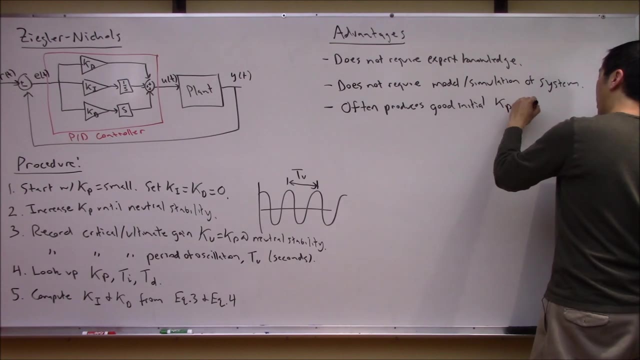 a good starting point for other techniques. So let's just write down that. another advantage is that it often produces a good initial Kp, Ki and Kd. right Again, that was the whole point of Ziegler-Nichols. 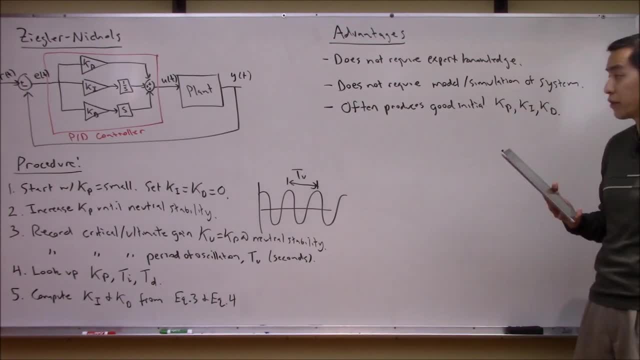 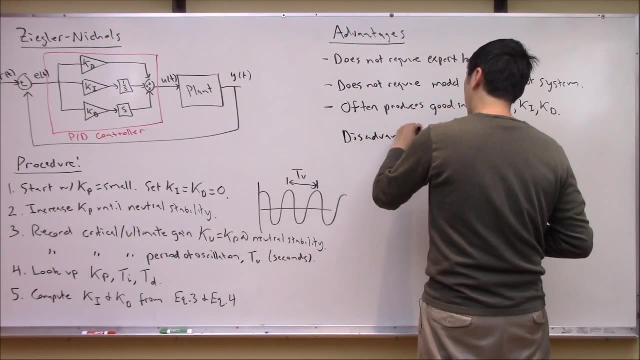 is just getting a reasonable point of our Kp, Ki and Kd that might work for your system. Okay, now those are some of the advantages. Let's talk about some of the disadvantages of this technique. Obviously, I think, probably the thing that's sticking. 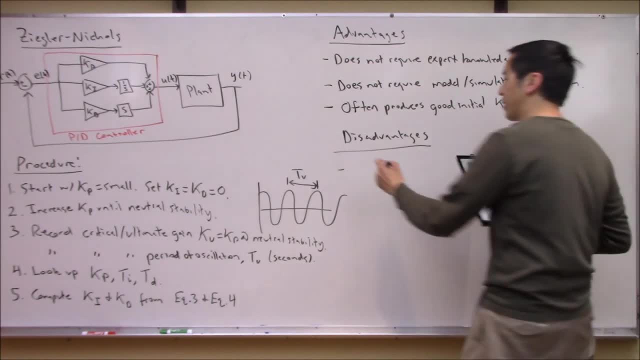 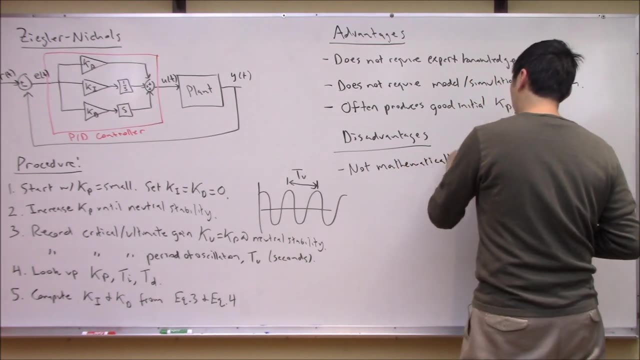 in the back of your head here is: it's not very mathematically robust here, So this is not- let's say not- mathematically rigorous, right? So there's no guarantee this is going to work for every system here. It works for a lot of systems. 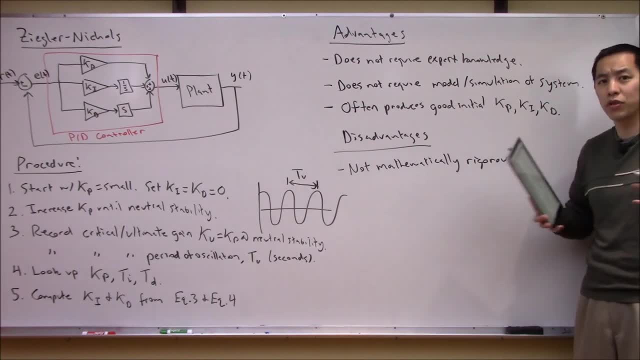 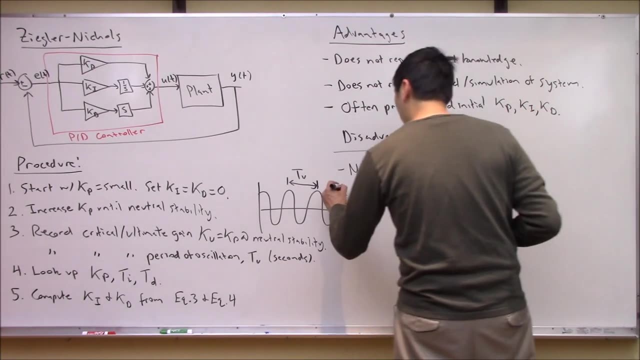 but I can't prove to you or guarantee that the poles are going to go to a certain location if I use this technique. The other thing is this requires- let me erase some of this a little bit so I don't spill over- If you look at the procedure, 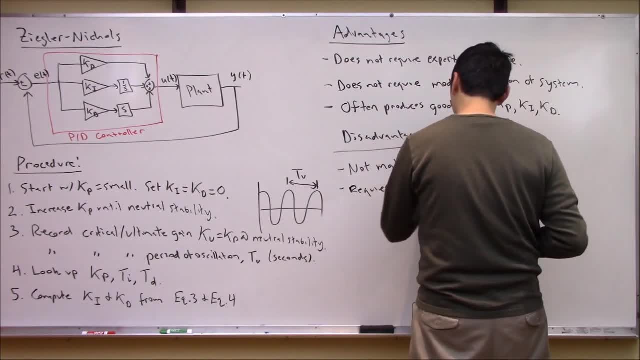 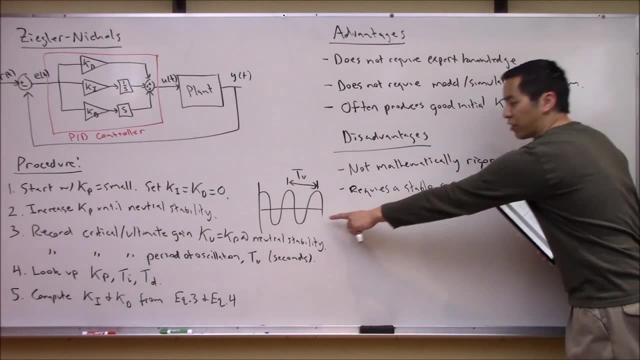 it requires a stable system. If your system was unstable to start with, there's no way you're even going to be able to perturb this and try to get this neutrally stable system, because it's just going to blow up the second you give it any perturbation. 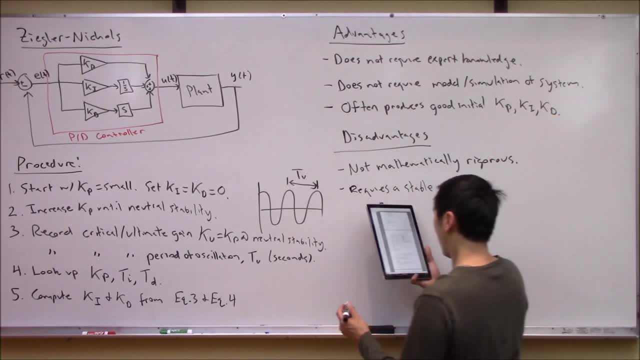 So you've got to start with a stable system in order to do this. What else is kind of interesting? Well, one thing that could be a disadvantage is if you don't have a model or a simulation of the system. it requires that you actually conduct this experiment. 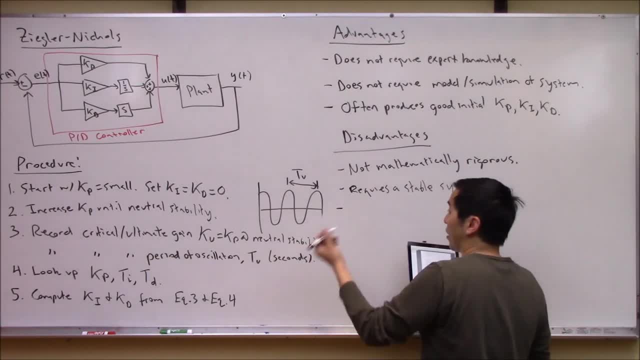 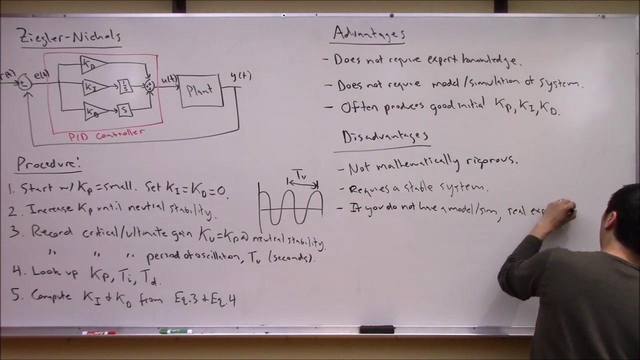 on the real hardware, which might be expensive. So let's just say, if you do not have a model slash simulation, real experiments could be costly. If this is your 747 aircraft and you're telling the company: hey, you know what I want to do. 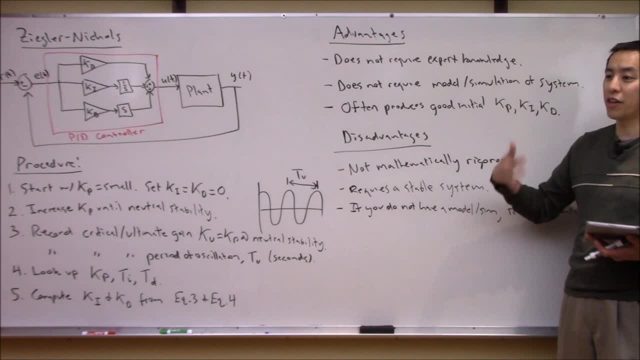 I want to go up there and I want to screw around with it and do a lot of these tests here and I want to change KP every single time and see when does the aircraft start pitching up and down? unstably, I bet you'd get laughed at. 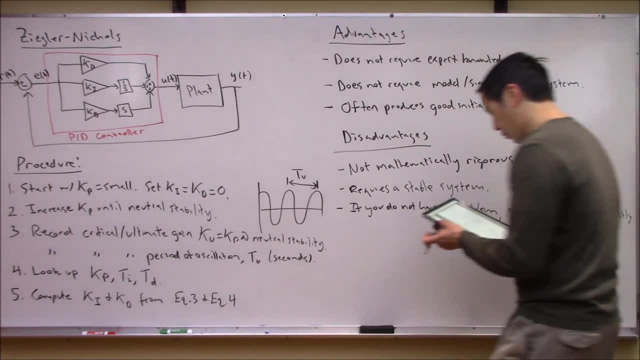 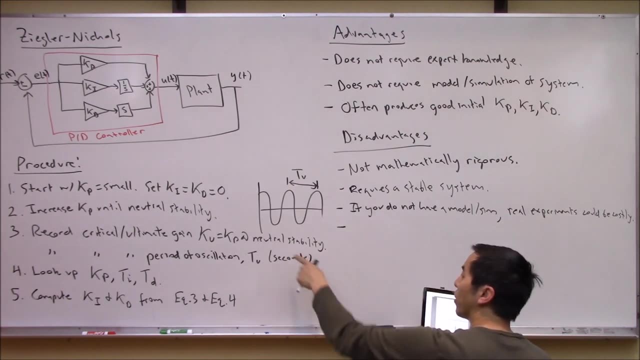 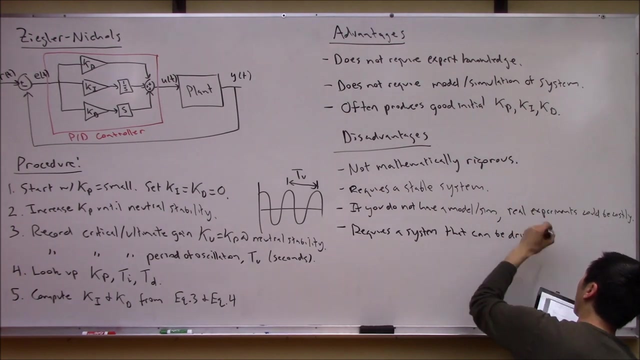 because doing that in real life is expensive and dangerous. The other thing that you might want to think about is also: it requires a system that you could actually drive to neutral stability. So let's just say it requires a system that can be driven. basically, I guess we could say: 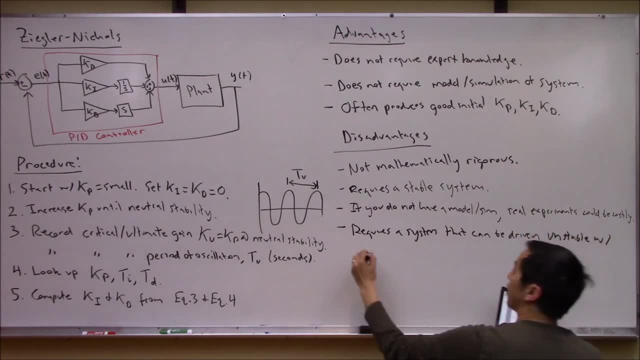 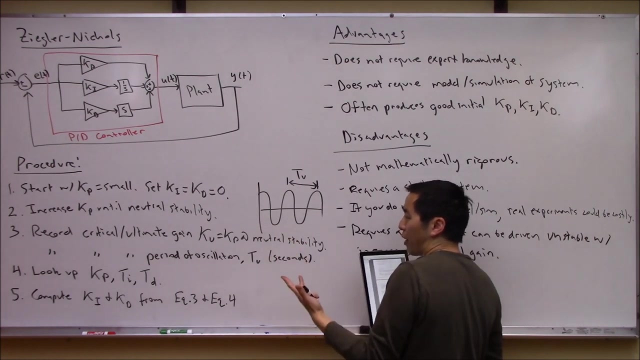 it can be driven unstable with increasing gain or increasing proportional gain, right, Because in order to get KU, we've got to get it to this situation where you have neutral stability. If you think about this long enough, neutral stability implies that what 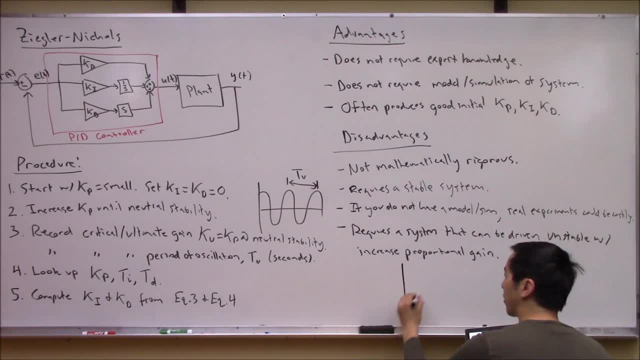 That some of the poles end up on the imaginary axis right. So if we look here at the real imaginary axis, I've got some system. I need to be able to drive it so that the root locus eventually starts to cross this. Well, what if you had a system that looked like? 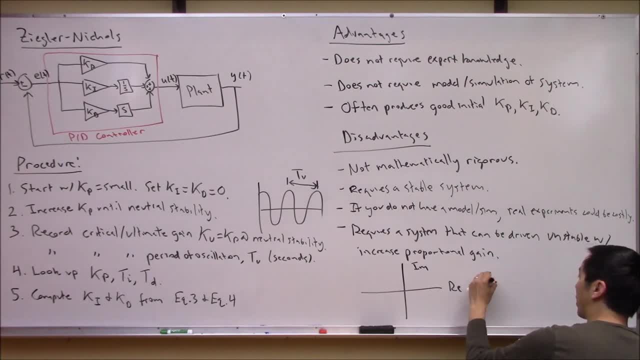 you know you could. for example, here's a counter example. how about G of S is one over S plus one right? That thing's just got a pole here at minus one right. What does the root locus for that system look like? 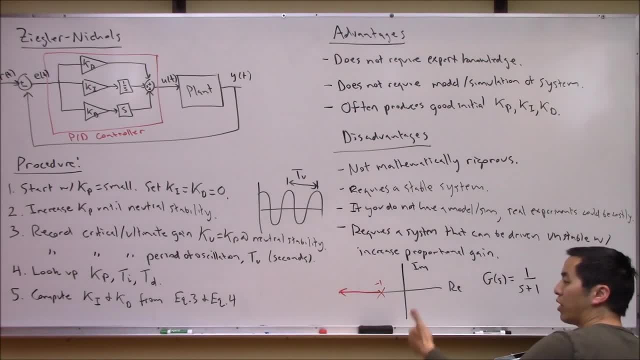 It is just this right. So as you keep jacking up, okay, this pole just keeps going further and further left, You'll never, ever get to the situation where you have these oscillations occurring. So in that case, this KU parameter is undefined. 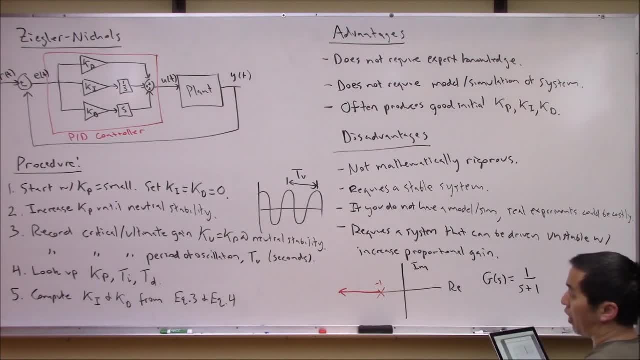 So, yeah, I think that's a pretty good discussion on the procedures, along with some of the pros and cons. Why don't we jump into an example to start? We're actually going to look at two examples. Let's start off with a purely thought experiment. 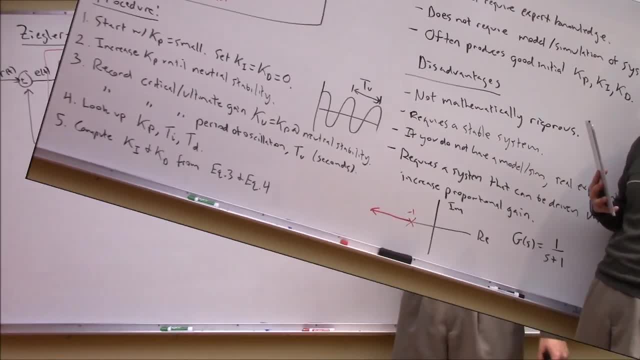 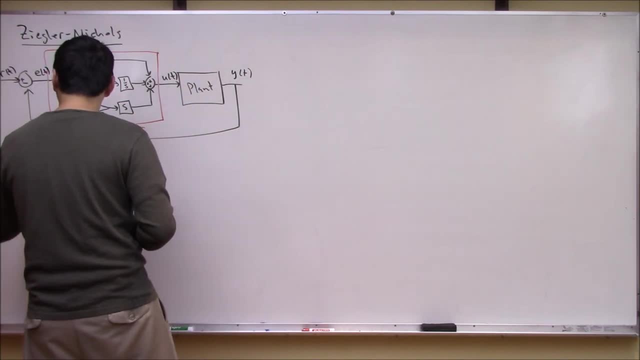 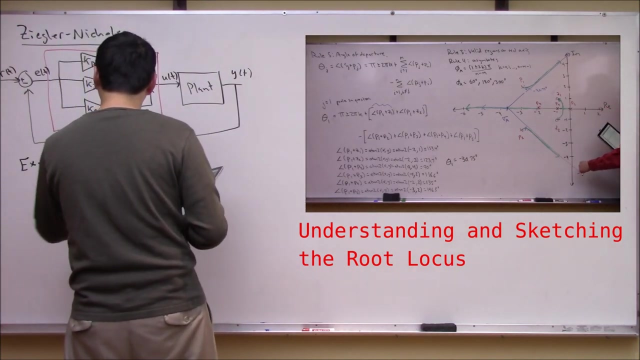 academic type example to start with. All right, So why don't we start with an example? This is actually a plant that we looked at before in our sketching the root locus discussion, So this here was a plant of one over S plus one. 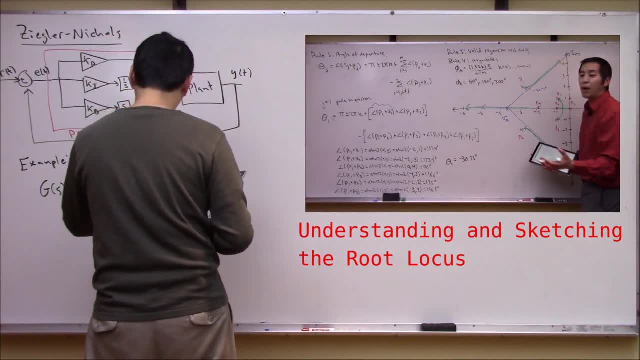 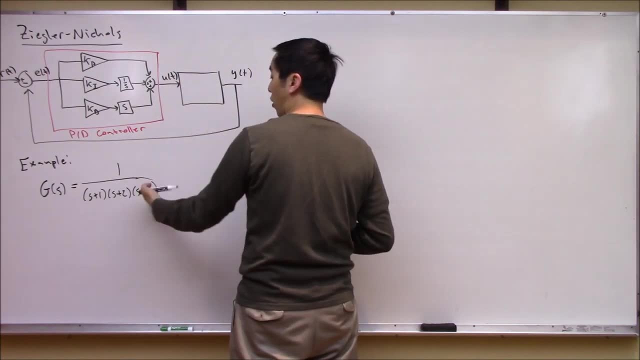 S plus two, S plus three, something really really simple. So in this case, instead of just having some generic plant, I now have a linear transfer function, ordinary differential equation, effectively representation of my system, And I want to go ahead. 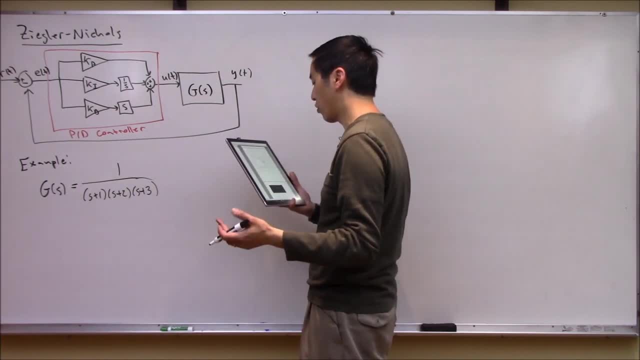 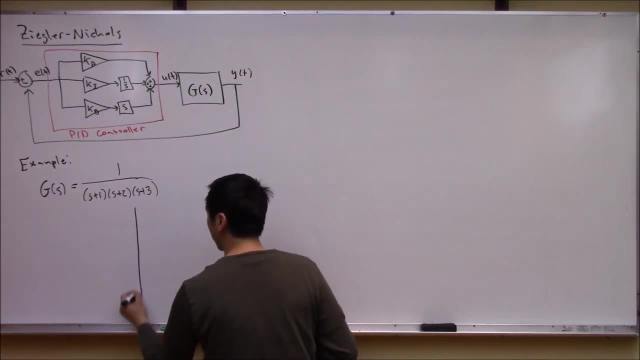 and try to find the KP, KI and KD values for this. Okay, So if you remember this system, let's go ahead and plot its poles, the open loop poles, on the real imaginary axis. I think this was really, really simple. 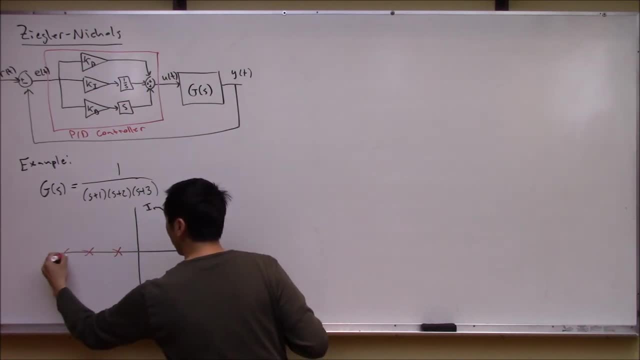 You got something here at minus one, minus two, minus three right, And if we wanted to look at what the root locus for this system looked like, it was something like: I think you got to the left here and then this pole is actually here. 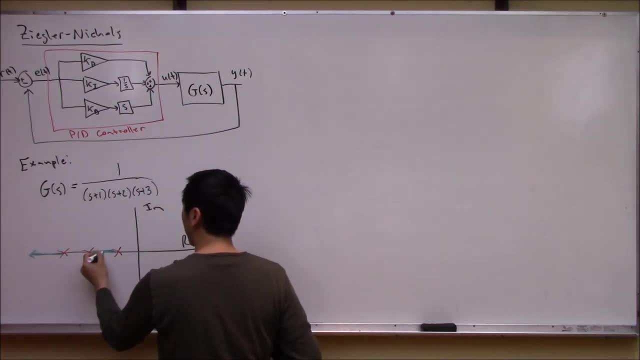 And then this pole is actually going out that way. These two are going to come together and then go off to asymptotes sort of here, I think at 60 degrees, and then something like this, right? So here's what the root locus looked like. 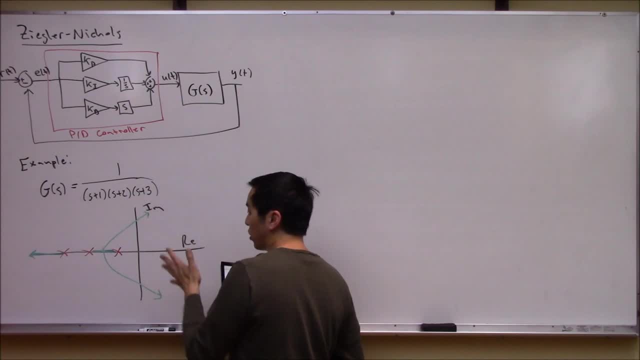 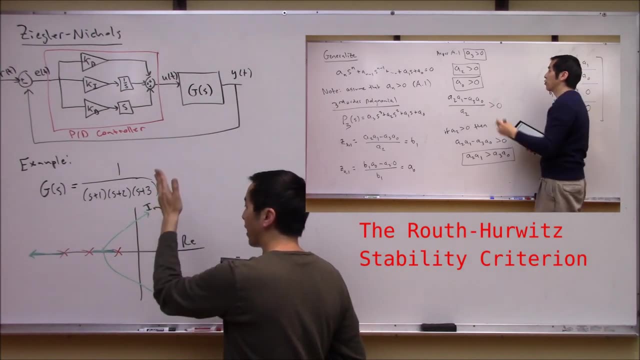 And in fact, in our discussion of sketching the root locus- as well as I think in our video on on Ralph Hurwitz actually is, you could actually use Ralph Hurwitz to find exactly the scenario we're looking for, right. 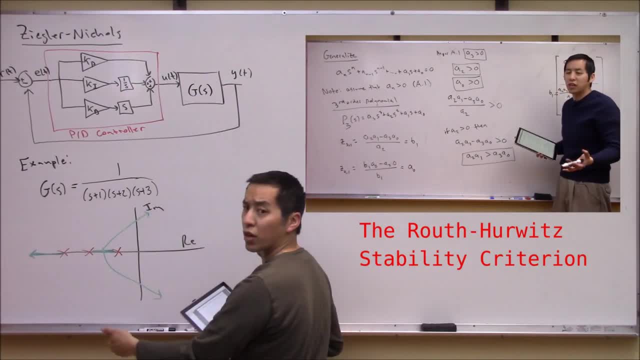 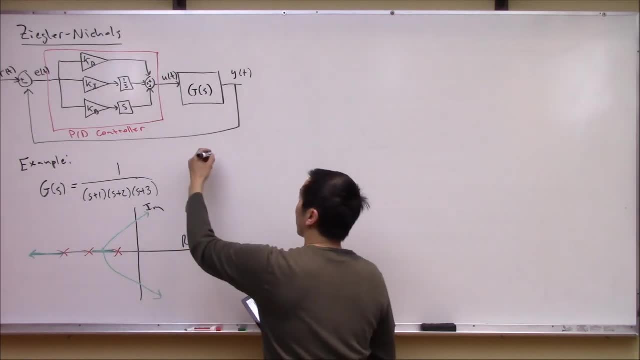 Because in all of these cases I want to look at where do some of these poles start crossing the imaginary axis Right. As soon as that happens, we have neutral stability. So with this system, what we could say is: let's go ahead and use Ralph Hurwitz. 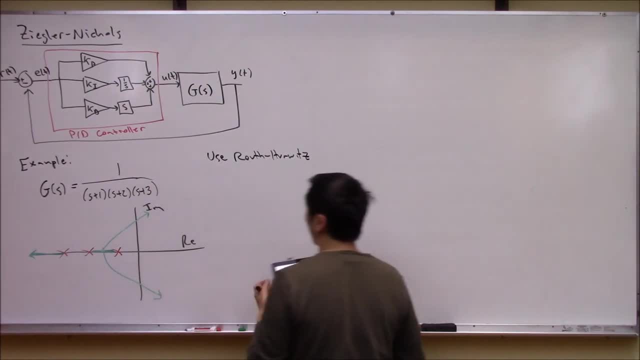 And in fact, again, this is the exact example I think we looked at in the Ralph Hurwitz video which is right over here. Feel free to refer to that video if you'd like to get this same solution, But I'm going to skip all of that. 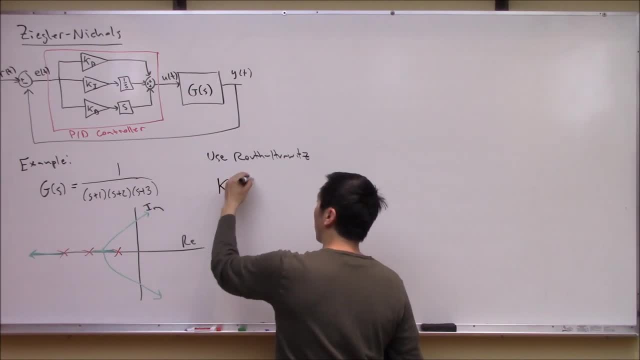 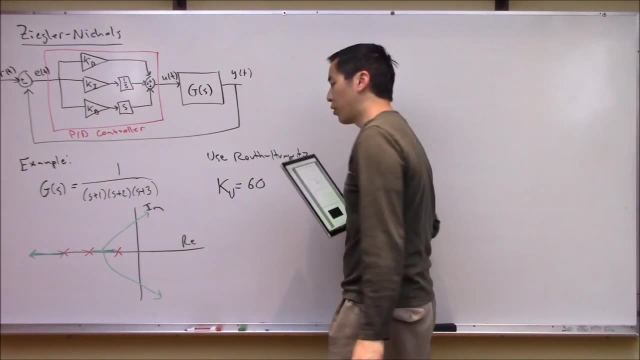 just because I'll assume you've seen that video already And we saw that a K of 60 over here, or I guess, a K of 60. I guess it's now KU. right, That's what we call is the ultimate gain. 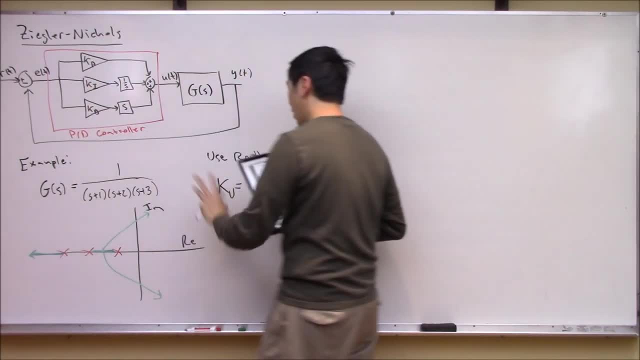 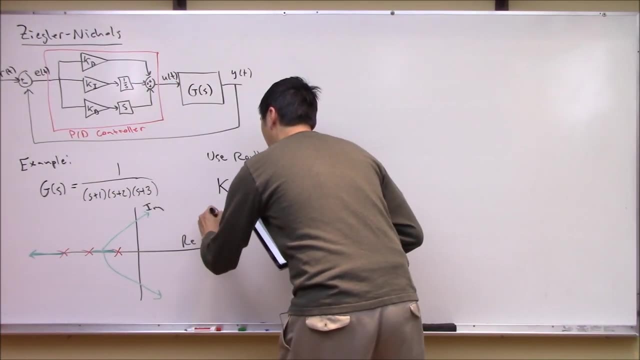 KU of 60, if I plug it in here, where these two is equal to zero, that will get us a neutrally stable system. So the next thing is we need to go ahead and find TU right. That was the period of oscillation. 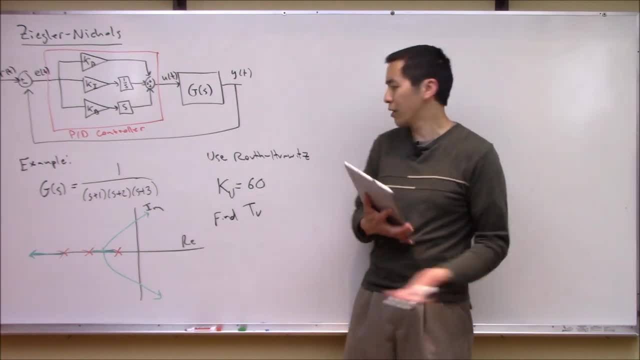 So in order to do that, what I think we should do is we should probably jump over to simulate and just heck, simulate this system where you've got this transfer function here for the plant and then a KP of 60 there. We'll look at the oscillations. 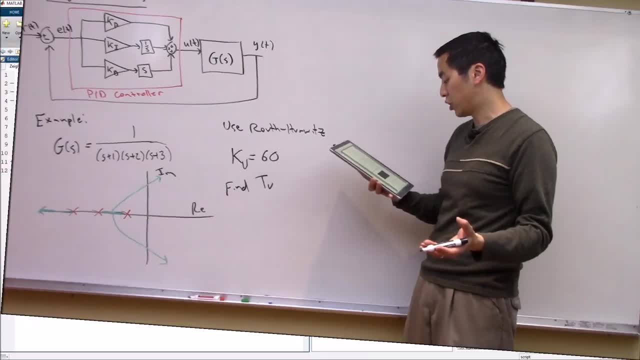 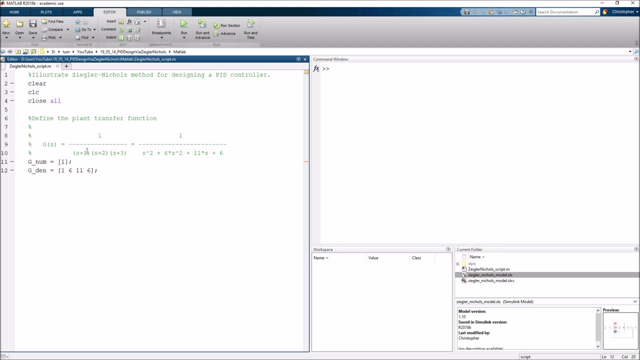 and we'll just directly measure the period from the simulation. All right, So here we are in MATLAB and I've already started a script, just so you don't have to watch me punch in all of this one line at a time. So the first thing we should do, 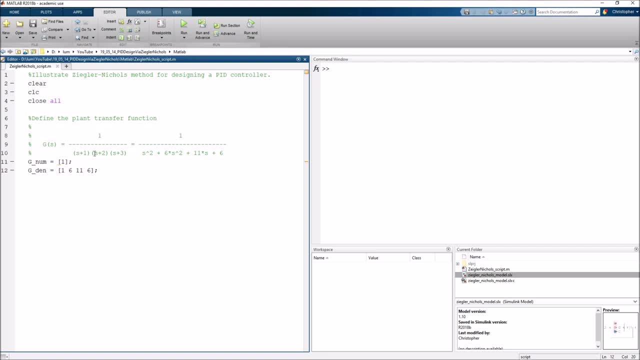 is, let's define the plant transfer function, which we said was 1 over s plus 1, s plus 2, s plus 3, which, when you expand out, you can write in polynomial format as such. Therefore, here's the numerator coefficient: 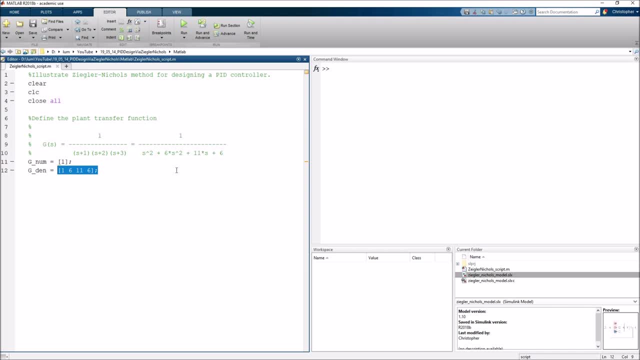 and the denominator coefficient vector to represent that transfer function. So let's just go ahead and run this to get gnum and gden into the workspace, All right? Also, to save us a little bit of time, I've already pre-built a Simulink model. 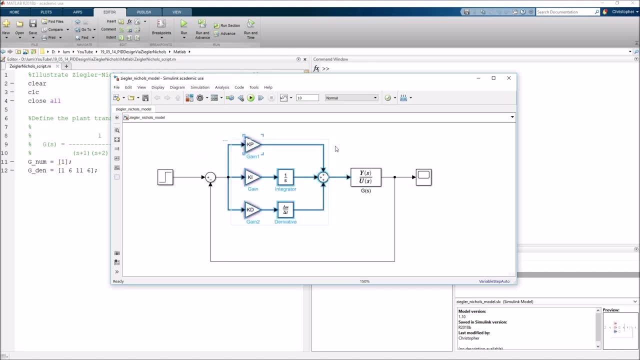 which has the plant controlled by our PID controller. Now we already know what the ultimate gain is from Ralph Hurwitz, but I thought it might be helpful just to pretend that this is a system where maybe we didn't know this and we want to walk through. 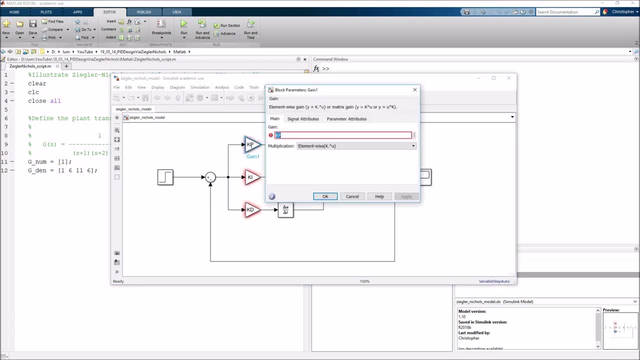 the full Ziegler-Nichols procedure. So we said the way we're going to do this is start off with a small kp, let's say 5, and we're going to set the other ki and kd to 0. And what we can do? 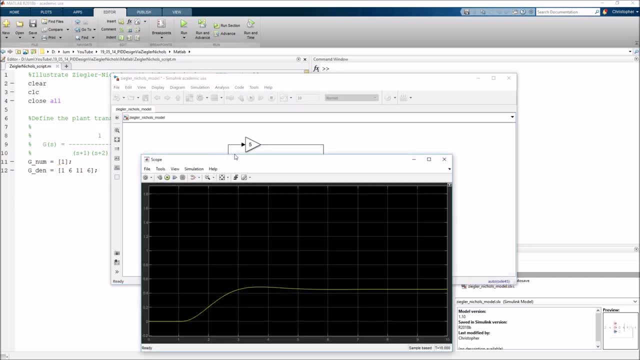 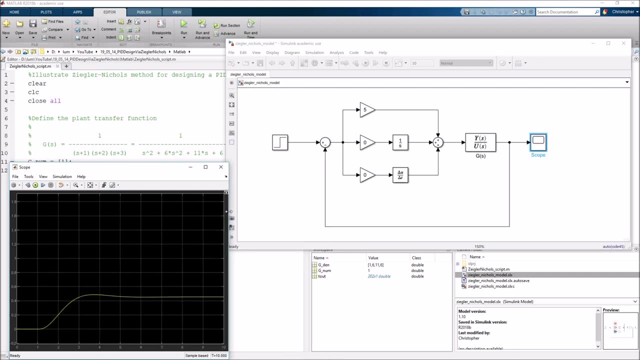 is just start running this simulation. So I'm going to run this and pull up the scope and we see: well, nope, that does not look neutrally stable yet. So let's keep on cranking up the kp gain. So let's go up to 25,. 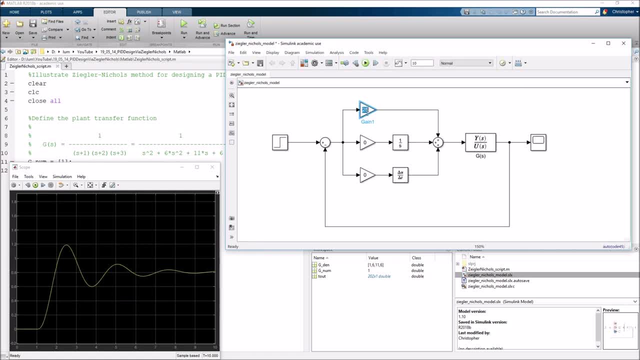 run this thing again and, yep, it's getting a little more oscillatory. How about 45?? Oop, that's looking better. And let's finally go up to 60, which we know should give us neutral stability. And yay, there we go. 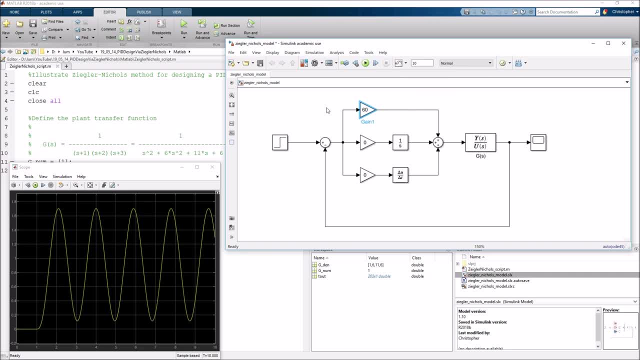 This thing looks neutrally stable, So we validated that ku of 60 is the ultimate gain we're looking for. So now all we need to do is just measure the period of these two waves. So you can see it's about two seconds. 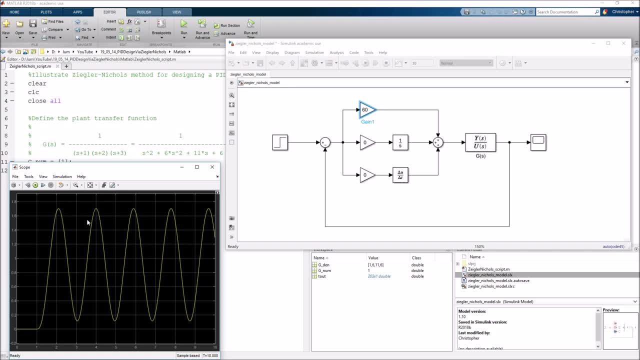 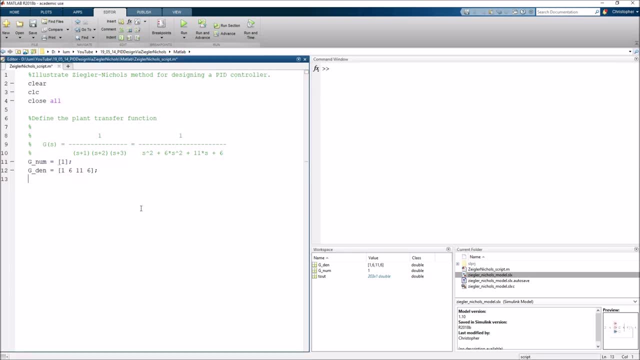 And actually, if you spend the time to zoom in and look at this, I think it's a little less than two seconds. I think we're using a value of 1.9 for the period. So, coming over to the script, let's just go ahead and define ku. 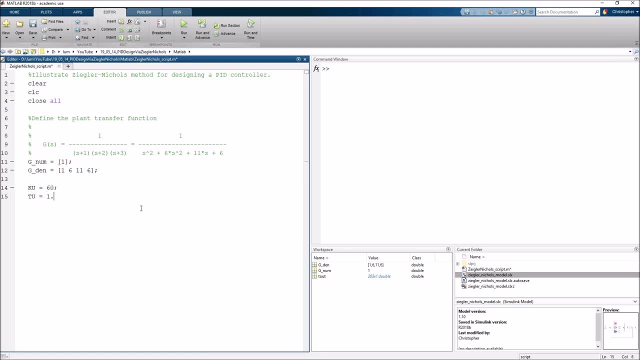 which we know is 60. And we now know tu is 1.9.. And we got the ku from Ralph Hurwitz, Or simulation, And we got the tu value from simulation. Okay, so the next step in the process is once we have ku and tu. 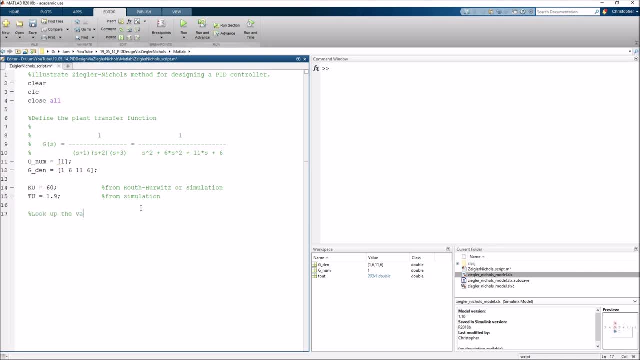 we're pretty much home free. We can go ahead and look up the valid or the appropriate value of kp, ti and td, right. So I think for this scenario where we are trying to do just a normal PID controller, we said kp was going to be 60% of ku. 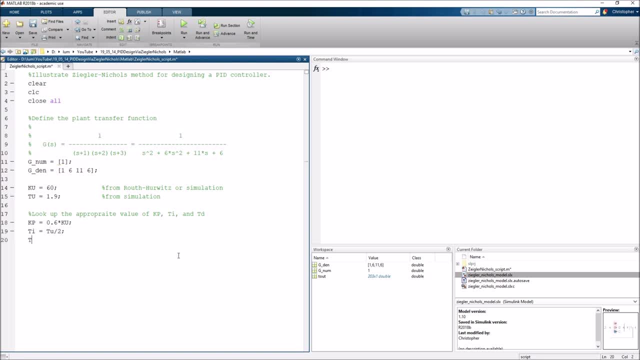 And then we said: ti was going to be tu divided by 2. And td was going to be tu divided by 8.. Great, So once we have those, we also said that you know you don't have to deal with these time constants, ti and td. 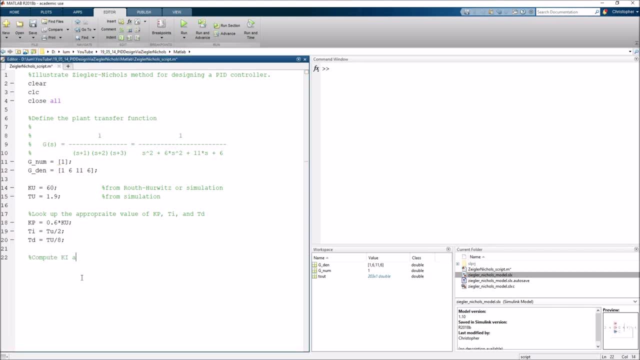 It might be more useful to compute now what the ki and kd values are using Again what we called equation 3 and equation 4.. So that was ki was kp, Ti was kp divided by ti, And then kd was going to be td times. 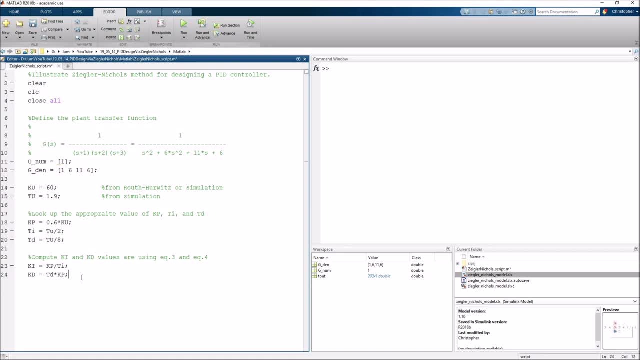 oops, t lowercase d times kp- Great. So if we run this, whoops, okay, I should have used the same variable, t, capital U There. we go All right There. So now we have a kp, a ki. 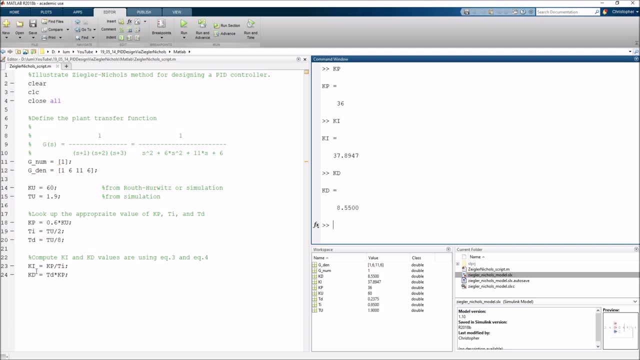 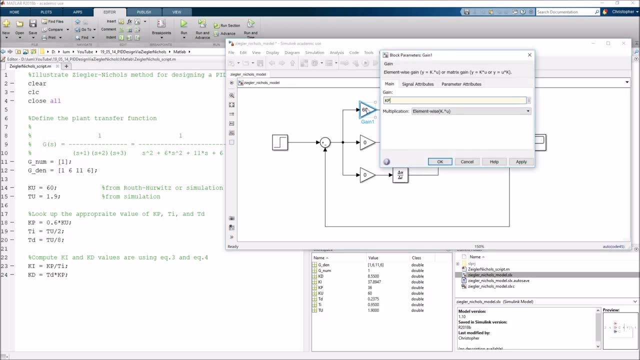 and a kd that was designed via Ziegler-Nichols. So if we come back to our Simulink model, we can see if that works. So let's go ahead and put in our kp, ki and kd. So go ahead and run this again. 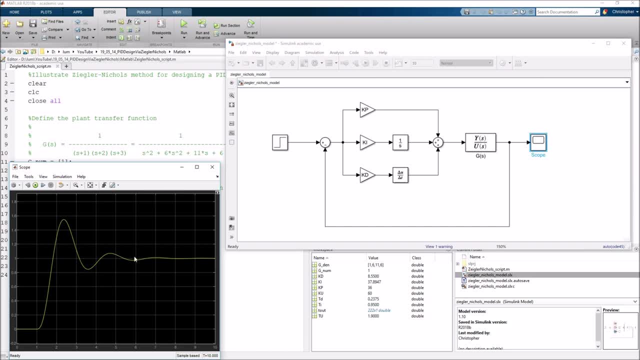 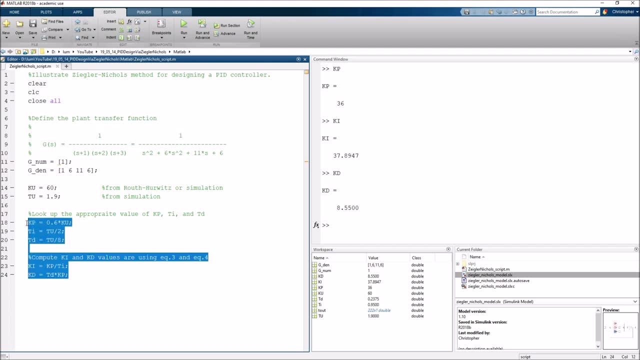 Look at the scope And look at that, We get a reasonable response. Just to maybe make a note of this: if you think about this long enough, all of this is just begging to be plugged into a function. This is basically a table lookup. 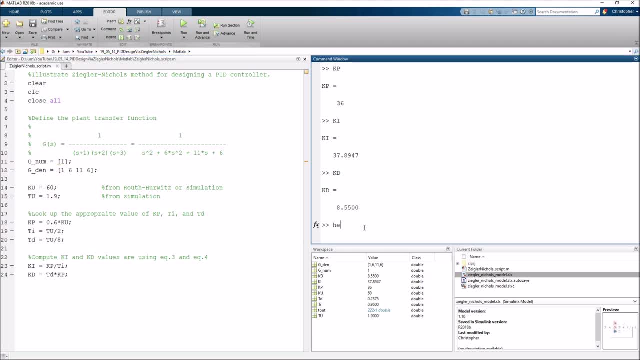 with a very simple calculation. So here's a little plug for my function that I ended up making called Ziegler-Nichols, which all this does is, if you think about it, Ziegler-Nichols- this whole procedure, right. 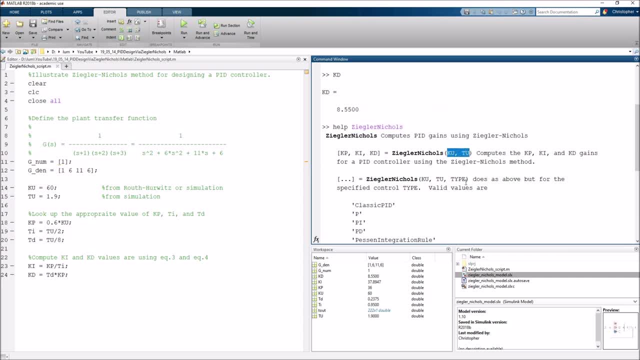 the only thing you need to know is ku and tu, And I guess you also need to know what type of controller are you looking to do. Are you trying to do classic PID? just a P, just a pi. pd, overshoot, no overshoot. 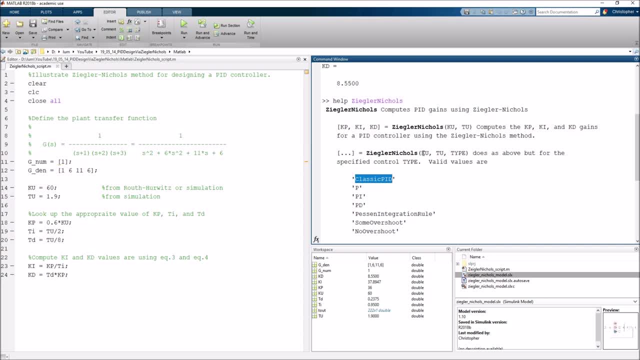 all of these different types. right, If you have those three pieces of information, you should be able to calculate kp, ki and kd with no problem. So what I've done is I've wrapped this into a function that I call Ziegler-Nichols. 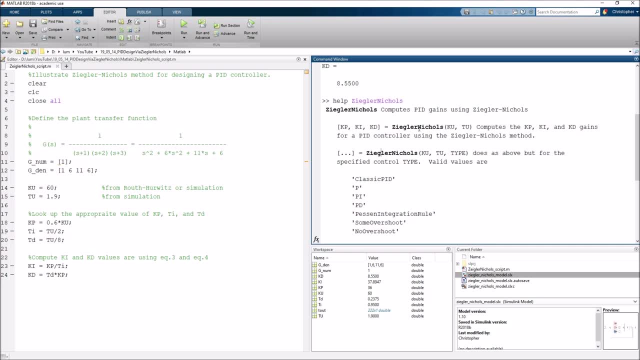 And I'll put a URL to this function so you can download it yourself. Surprisingly, I didn't find it natively in MATLAB. Maybe it is natively supported in MATLAB, Just so, please shoot me a message or leave a comment down below so we can all learn. 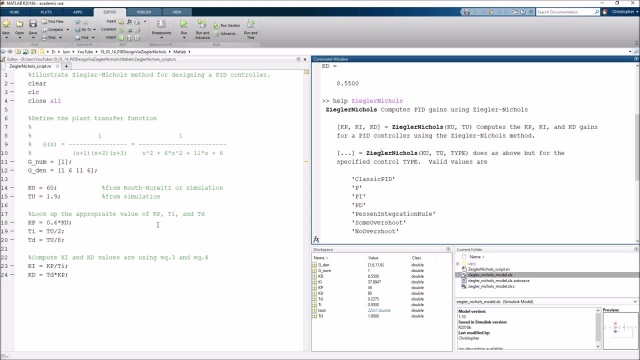 But I ended up just coding this up in a couple of minutes and I thought I would share this with you guys. So, alternatively, what you could do is let's just use the custom Ziegler-Nichols Ziegler-Nichols function. 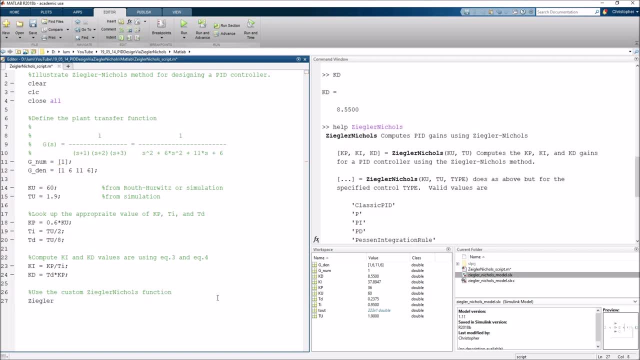 All right. so the other thing we could do is just call the custom Ziegler-Nichols function and you pass it ku and tu, and maybe let's say we want to do classic pid, And what my function will easily compute for you is just the kp, ki and kd gains that are necessary. 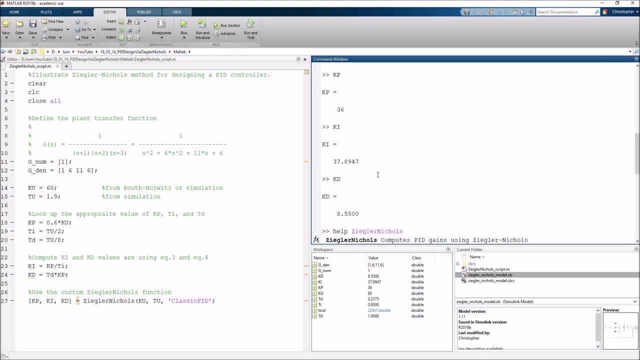 Now, before we run this, maybe what we should do is let's scroll back up and see what we got earlier, Right? And then we manually computed them: Okay, 36,, 37.9, and 8.55.. So now, if we were to run this script, 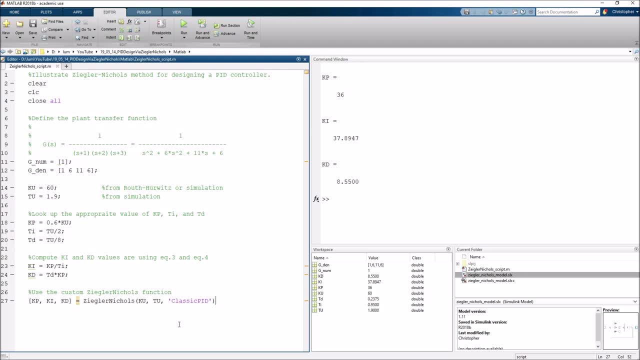 you see that we basically get the exact same values. So the nice thing about the Ziegler-Nichols function that I provided is that it supports not just, like we said, not just classic pid. but what if you wanted to do just? 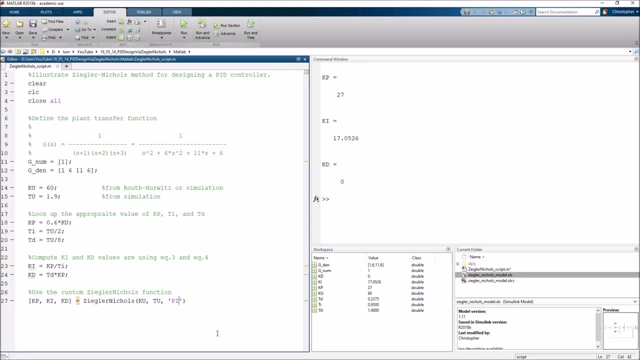 sorry, not just classic pid. but if you want to do something simple like just pi, you could get another set of gains or you could do like no overshoot And get yet another set of gains. So I think it's pretty helpful so you don't have to do that manual table lookup. 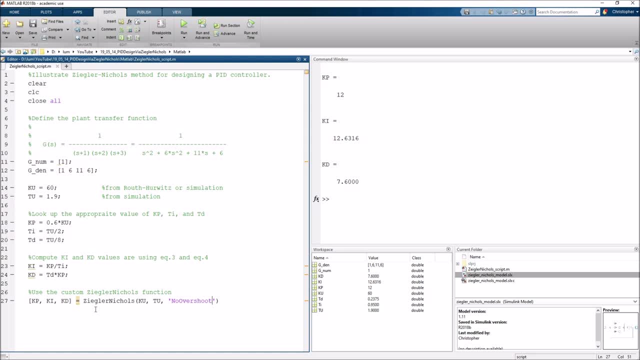 and calculation by yourself. So again, there's a URL to download this in the description of the video. What might be helpful now is let me flash up a picture that shows the system response using a bunch of different sets of gains for all these different conditions like: 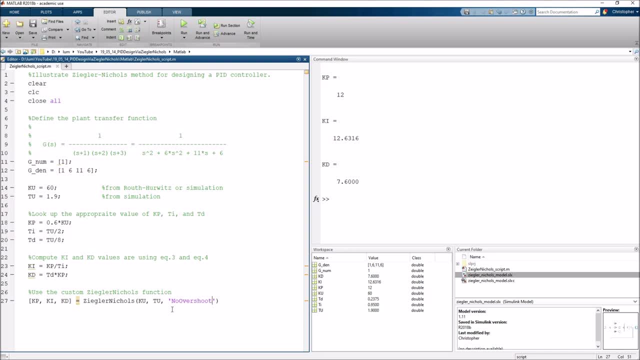 classic pid pi, no overshoot, etc. Just so we can get a feel for how the system behaves and to make sure that the Ziegler-Nichols technique gets us a reasonable controller for this system. All right, so here's a MATLAB figure. 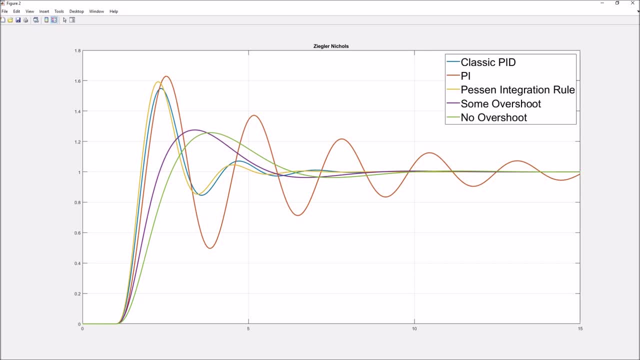 that is basically the simulation we were just running here, but just using all of those different permutations of pid controllers that were derived using Ziegler-Nichols and these different types of methods. So, as you can see, they all give you know. 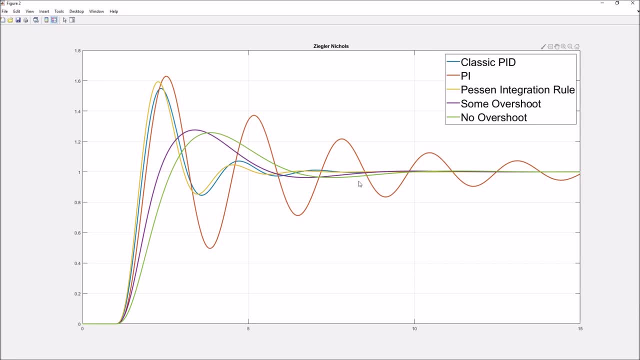 halfway reasonable responses. They all look like they're tracking to the desired reference, with zero steady state error And, as you can see, some of these things where, if you want, maybe some overshoot or no overshoot, like these green and purple lines, 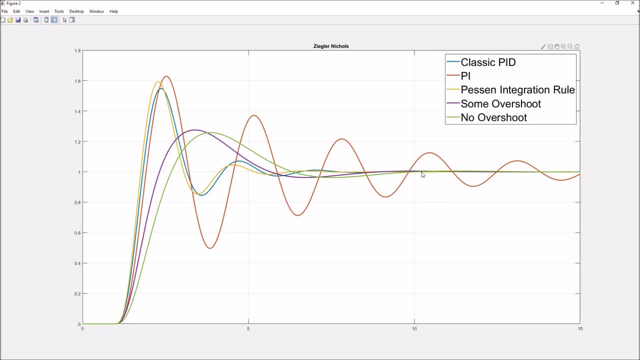 they do seem to follow that behavior in general. So this is sort of a heuristic, anecdotal example showing the viability of using Ziegler-Nichols to design a control system for a situation where you've got a nice mathematical plant model already sitting there waiting for you. 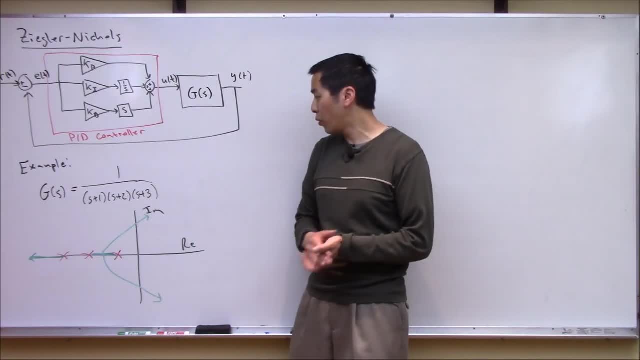 All right. so we saw that Ziegler-Nichols worked pretty well for designing a pid model. We saw that Ziegler-Nichols worked pretty well for designing a pid controller for this transfer function. But actually, you know, if you think about this long enough, 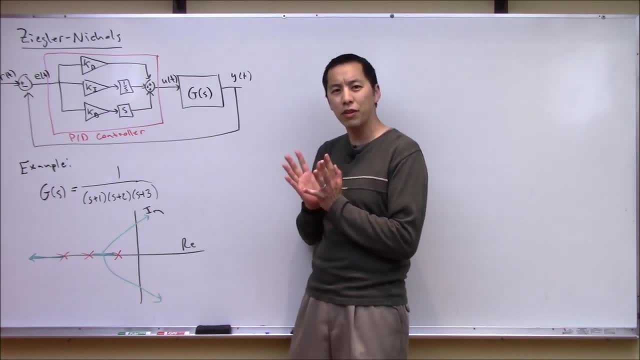 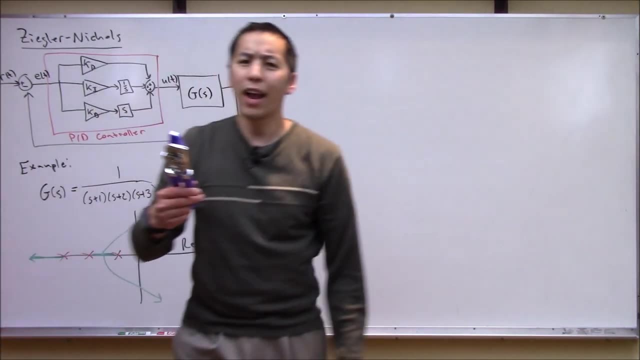 if you've already got a mathematical model of the system and you're using Ziegler-Nichols, I kind of think you're doing it a little bit wrong. It's almost like you've got a can opener And instead of using the nice normal way, 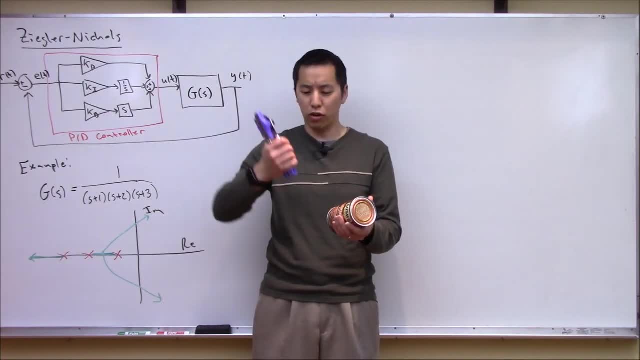 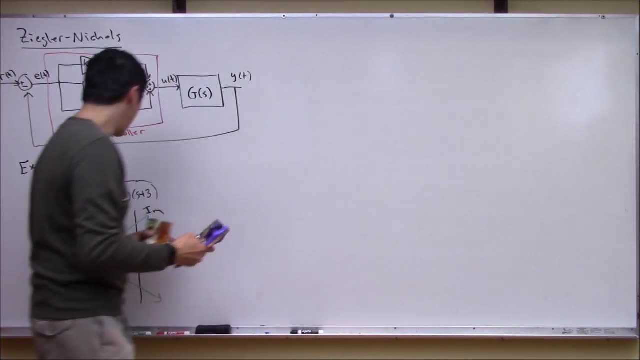 and the proper way of opening the can with the can opener. you're going to sit here and you're going to try to bash the can open with the handle of the can opener. There are better ways to design pid controllers for systems where you already have. 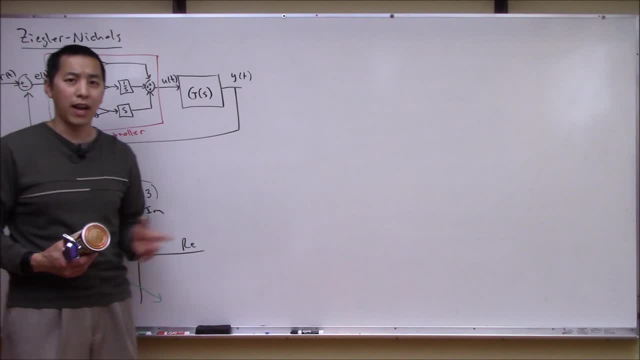 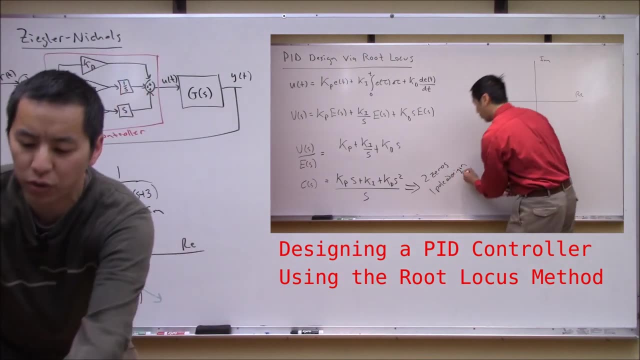 a mathematical model of the system And, in fact, we're going to look at that in a couple of these other videos where we talk about using root locus to design it. Now, that being said, Ziegler-Nichols, in my opinion, 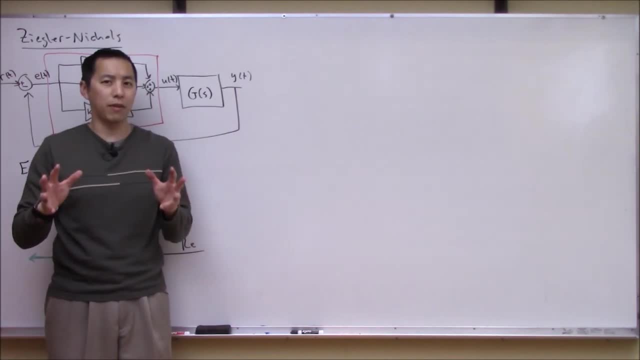 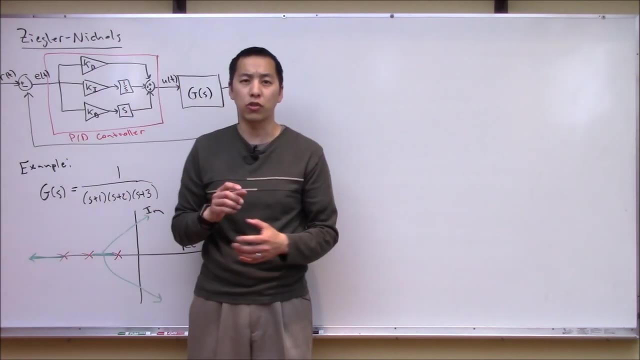 one of the places where it really shows its versatility and power is where you want to design a pid controller directly with an experimental system, without ever needing to develop a transfer function or a simulation of the system. You're going to want to do this iteratively and online. 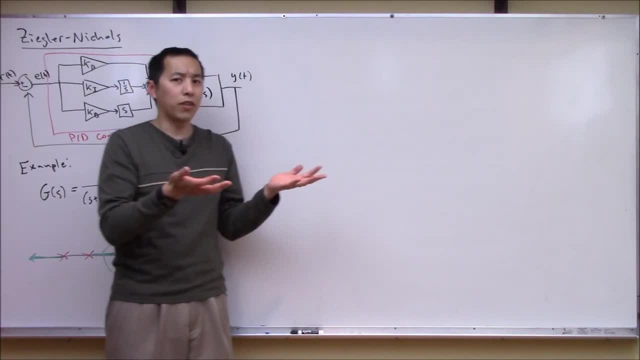 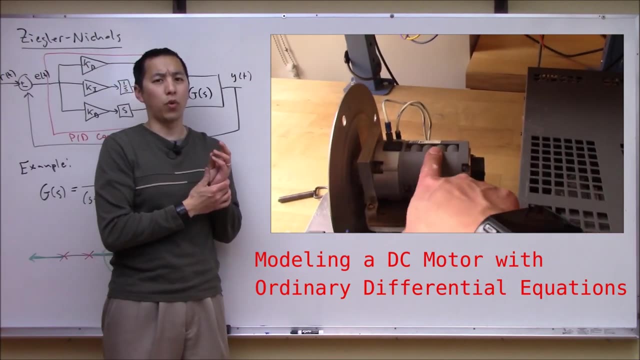 So the example I'd like to look at now is: let's walk over to the lab and see if we can design a pid controller for a DC motor, And, if you remember, we talked about developing models for a DC motor in some of our other videos. 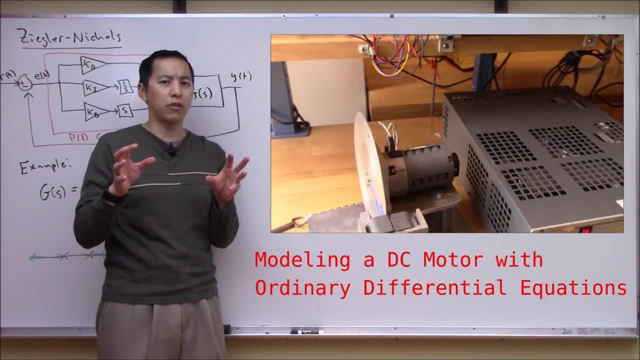 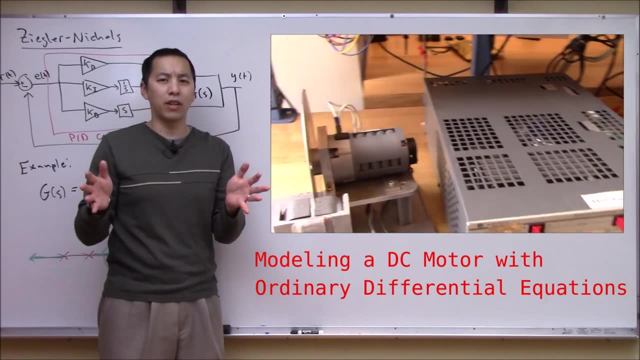 But again, the hat I want you to put on right now is: think about what if we didn't have these models here of the DC motor? And we have a system that I can play with. Let's see if we can just go into the lab and see. 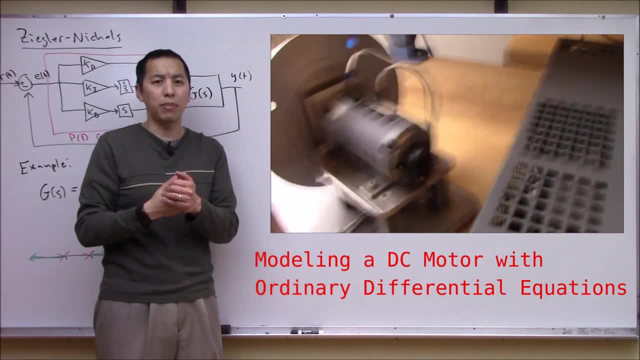 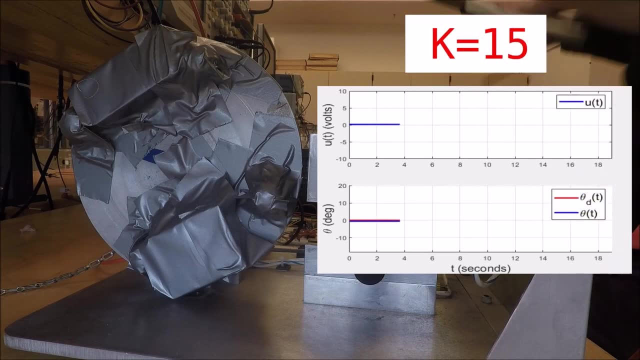 does Ziegler-Nichols allow us to synthesize a pid controller for that system Iteratively and online? Let's start with a proportional gain of 15.. The constant reference signal is simply 0 degrees. so when we introduce some error by manually disturbing the wheel, 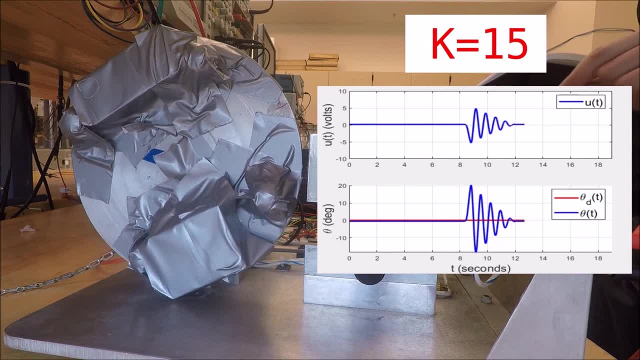 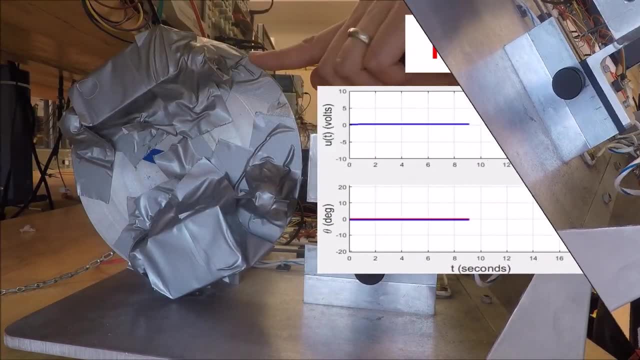 the system attempts to return to 0.. As you can see, there's a few oscillations, but for the most part the system response is more limp than a wet noodle because the gain is relatively low. Alright, so let's bump up K to 25 and try again. 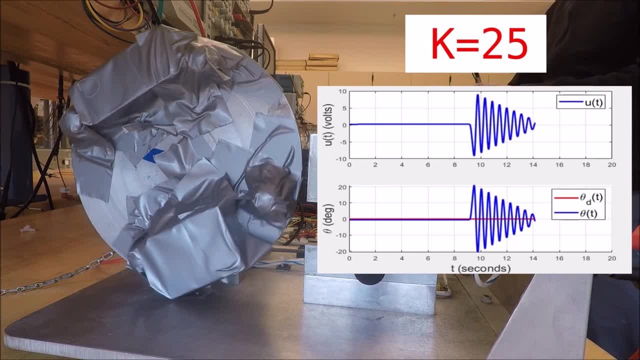 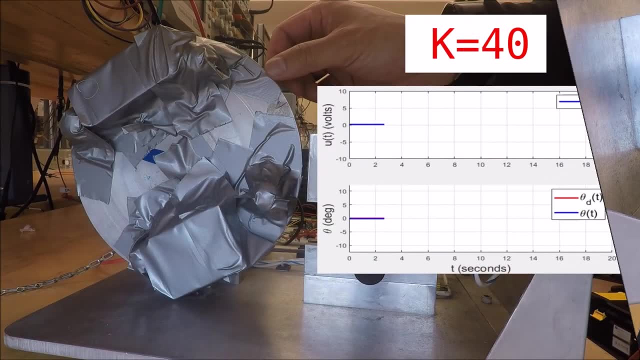 And, as you can see, we're definitely moving in the right direction. The oscillations are increasing, although the system is still reasonably stable, so we're not quite there yet. Alright, so let's increase K to 40 and try again. 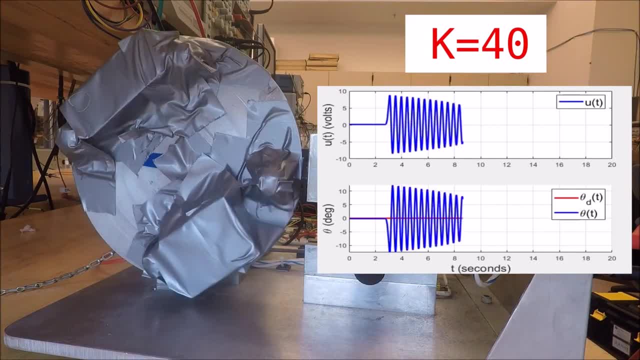 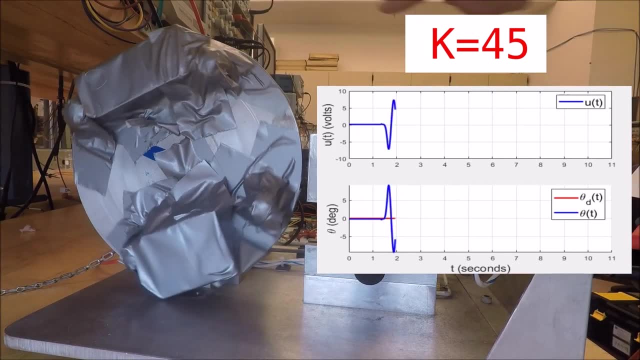 And- oh, that's close, but no cigar- You can see that the system is still barely stable, So we just need to push it a little bit harder. So let's increase the gain again up to 45, and now it looks like we've finally pushed the system. 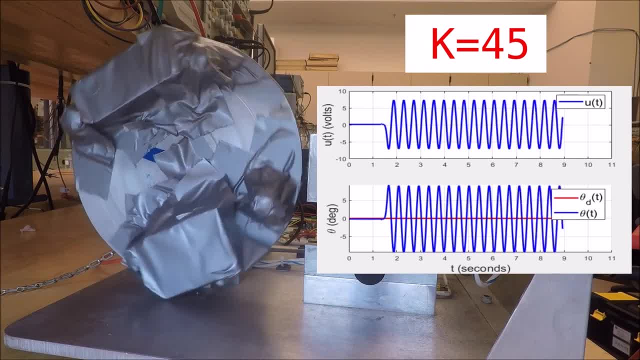 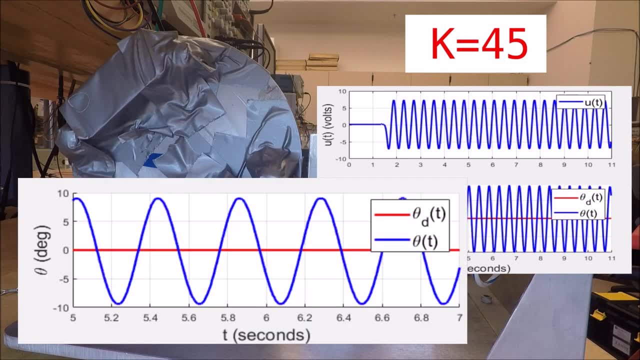 to neutral stability, as evidenced by the persistent oscillations at constant amplitude. So now we know that Ku is equal to 45.. To get Tu, let's just zoom into a section of this trace and then simply measure the period of the oscillation. 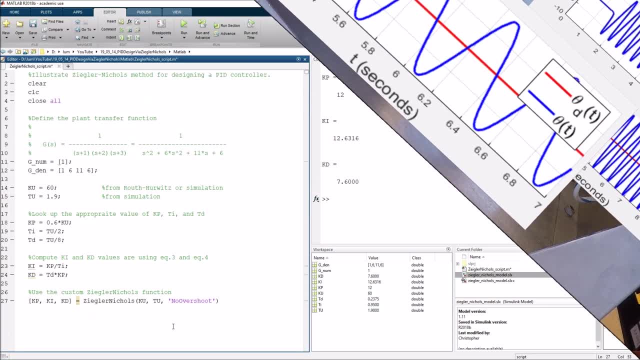 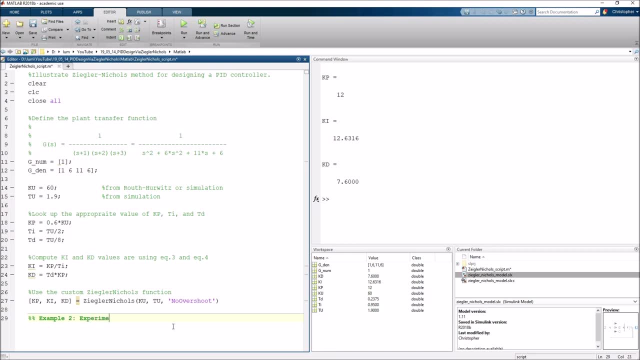 which appears to be around 0.96 seconds. Alright, so let's run back to MATLAB and maybe we'll start a new section. Let's call it Example 2, Experimental DC Motor. And now it's really just a simple matter of. 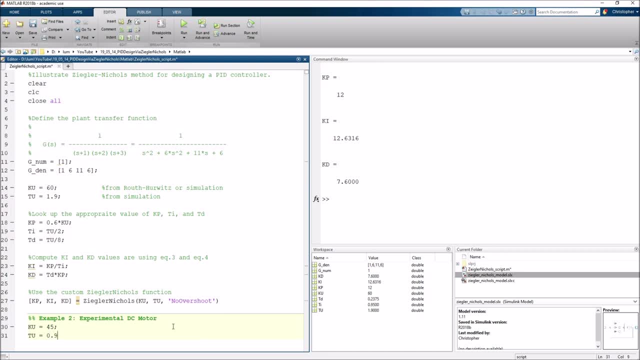 inputting our Ku and Tu values that we obtained in the lab and then doing the Ziegler-Nichols lookup slash calculation. And again, to save myself the busy work, I'm going to use my custom-made Ziegler-Nichols function. 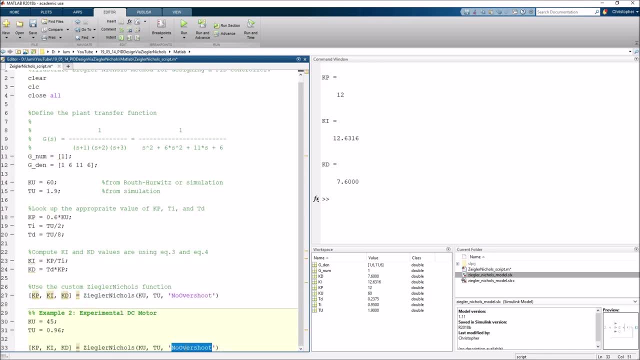 And we are going to do. Let's do this with Classic PID, how about? And just re-running the script? now we get a new set of gains that are tuned for this specific system. So why don't we run back to the lab? 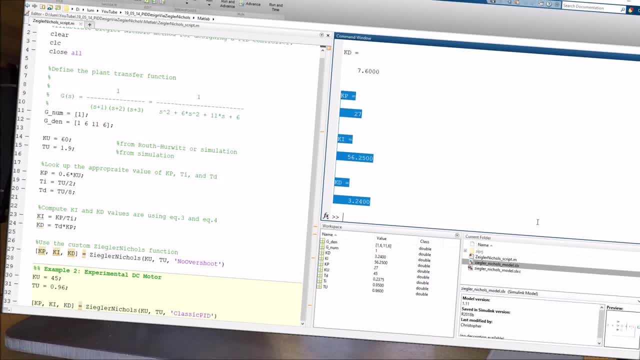 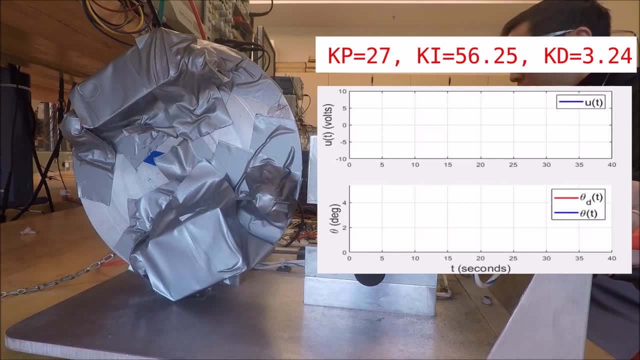 and see how these set of gains perform on the real DC motor system. So in this case we're going to command a step change in motor position. When the step is introduced, pay attention to both the system output, which is the motor position. 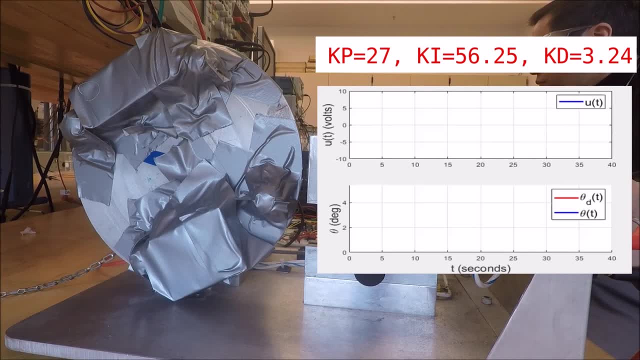 and the control signal, which is the voltage to the motor. So in this case we use a step from 0 to 0.09 radians, which is about 5 degrees. We use a small deflection in an attempt to avoid controller saturation. 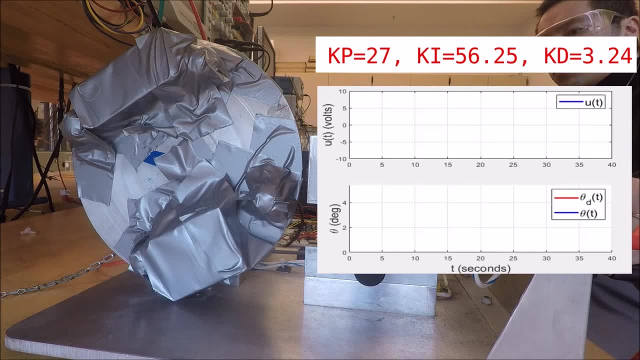 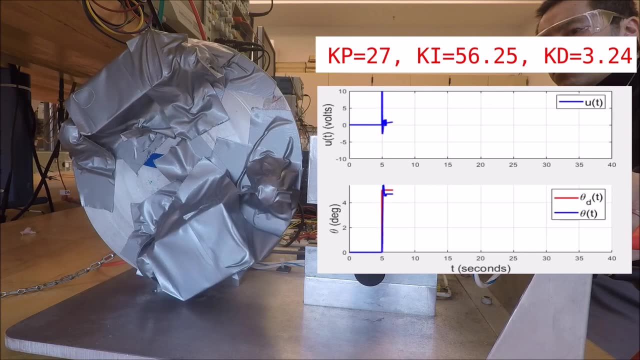 The power supply in our experiment can only supply plus or minus 10 volts. Despite our small step magnitude. the controller requests 30 volts. I've adjusted the axis of the plot to plus or minus 10 volts so the scale isn't blown out of proportion by this spike. 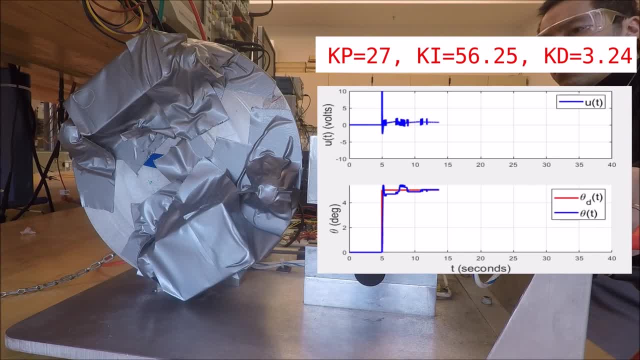 When the controller saturates. the Ziegler-Nichols designed PID controller is effectively acting non-linearly, so all bets are off. While we're talking about non-linearities, we should probably mention that another source of significant non-linearity in the system, 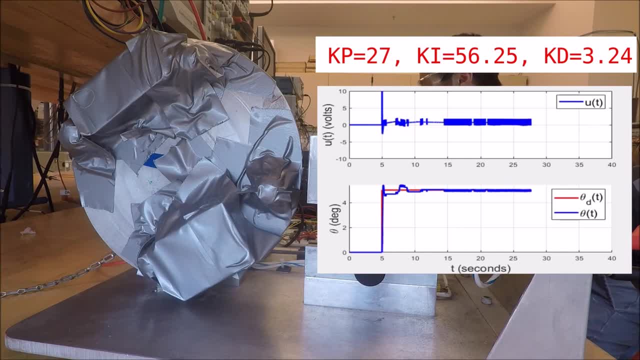 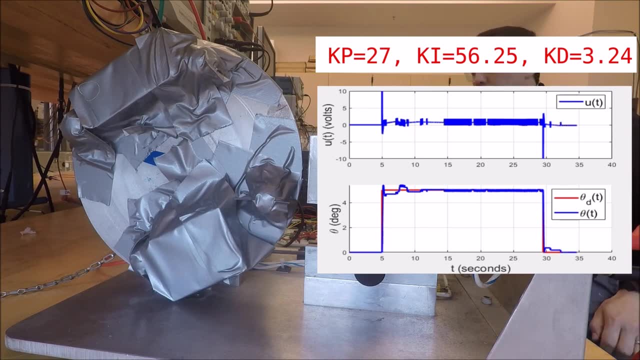 is the friction. You've got viscous friction, Coulomb friction and stiction, all acting on the system. These non-linearities are most predominant in the system and that's exactly where we're operating, Combining this with the finite resolution. 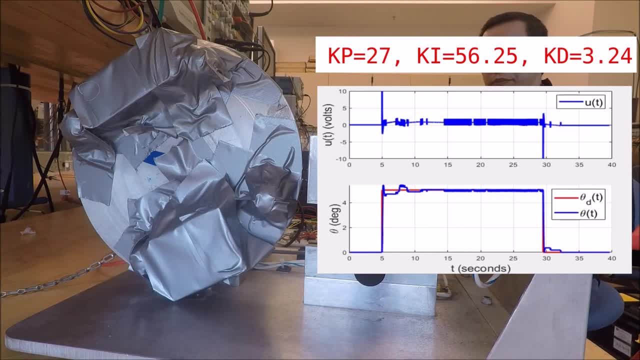 of the position encoder explains some of these jitters you're seeing in the position and therefore in the control signal as well. We do get a little bit more lucky when we do the step back to 0 degrees. Despite all of these non-linear effects. 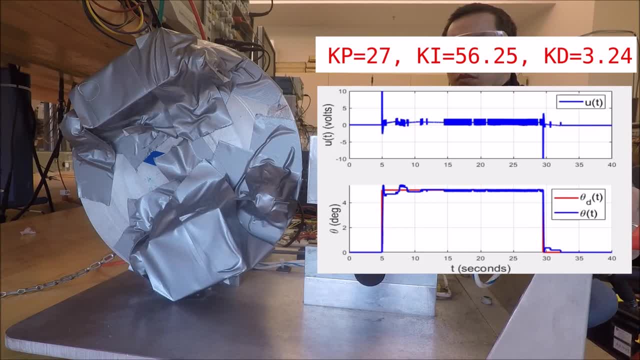 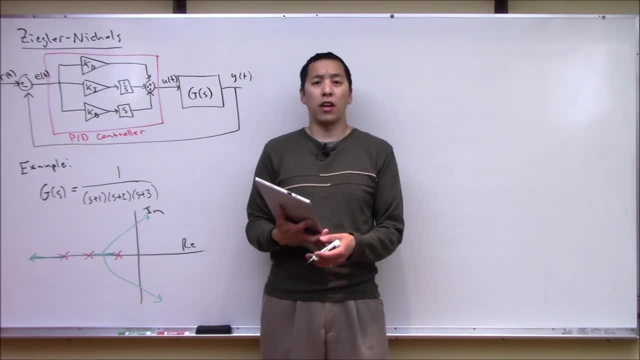 we see that the PID controller does its job respectably and actually works quite well for this system. Alright, so hopefully that convinces you that Ziegler-Nichols is a reasonable way to go about designing a PID controller for a system either where you have a model of it. 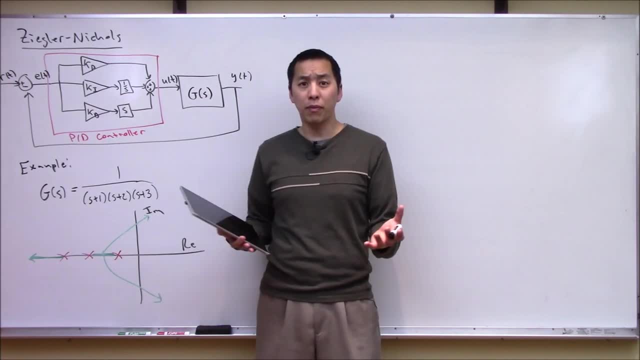 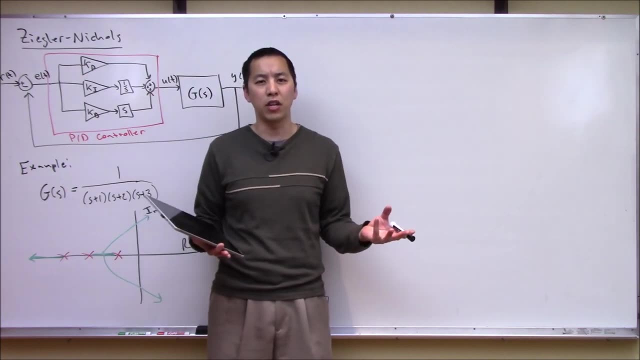 or you don't. So, that being said, I think that wraps up the discussion today. I hope you'll join us at a future video where we're actually going to continue our discussion on PID controllers and look at other ways to synthesize PID controllers.